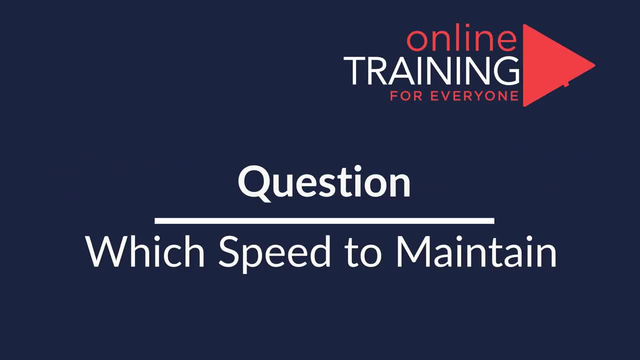 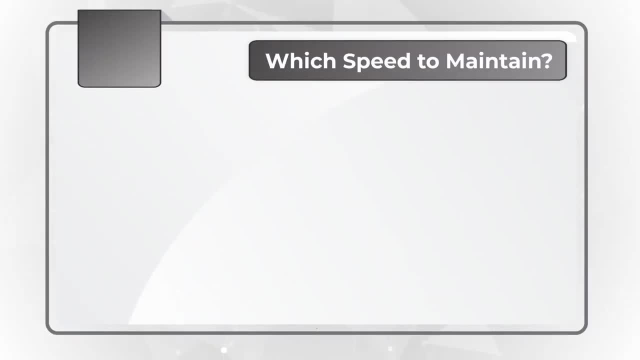 Let's look at the very interesting question which tests your math skills as well as your logical reasoning skills. You need to determine which speed should Anisha maintain? Usually when running, Anisha covers 8 miles in 15 minutes. Today she covered 3 mile distance in 2 fifths. 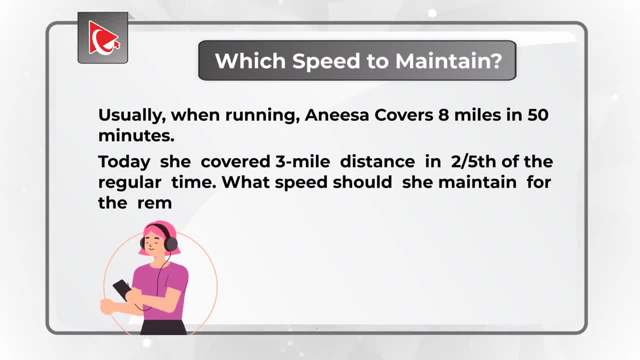 of the regular time. What speed should she maintain for the remaining distance to cover it in the regular time? And you're presented with four different choices to choose from: Choice A- 8 miles per hour, Choice B- 10 miles per hour, Choice C- 15 miles per hour, And then 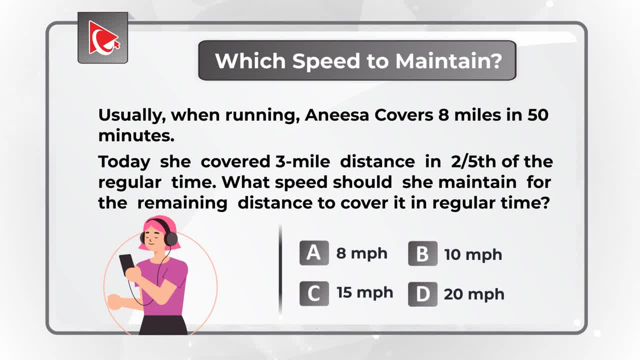 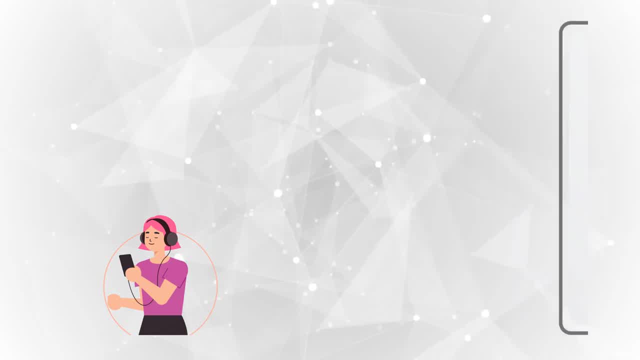 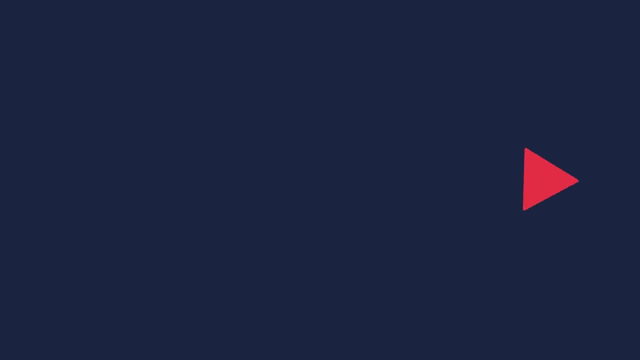 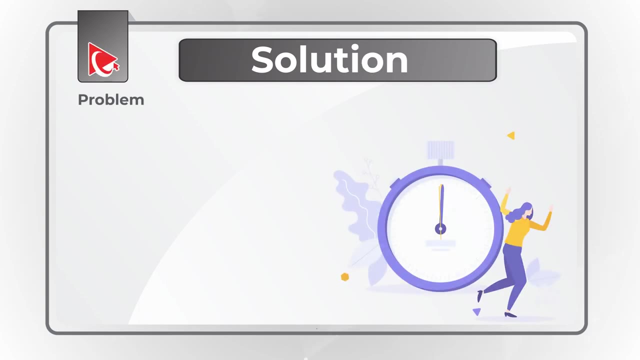 choice D: 20 miles per hour. Do you know the answer? Give yourself a little bit of time. maybe pause this video to see if you can come up with the solution. Are you ready? Let's move forward and get started. We only have two facts in this problem. Total distance equals 8 miles per hour. 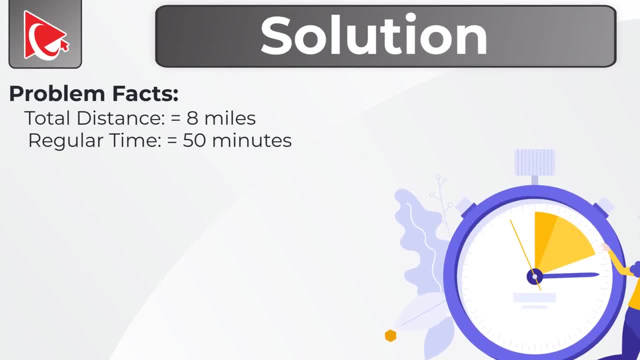 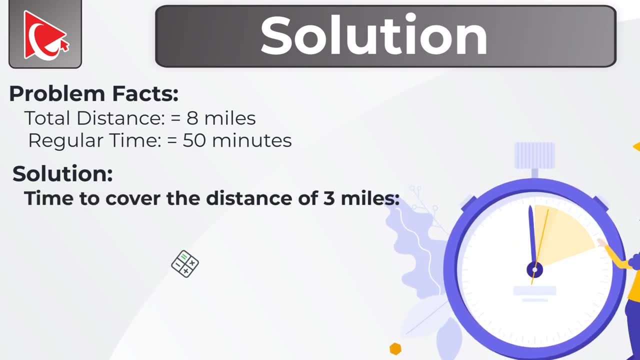 And regular time Anisha covers this distance is 50 minutes. So to get to the solution, we need to determine time to cover the distance of 3 miles. Let's first calculate how long it took for Anisha to cover the distance of 3 miles. 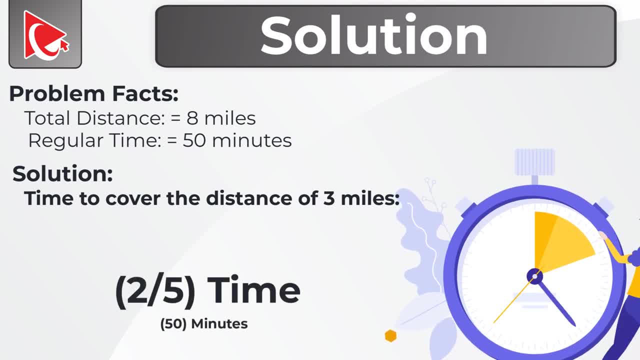 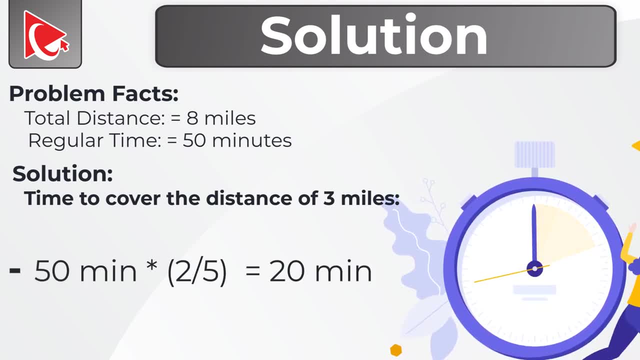 We know that it took her 2 fifths of the regular time, And regular time is 50 minutes. To calculate it, we need to multiply 50 minutes by 2 fifths, which would equal 20 minutes. We know that it took her. 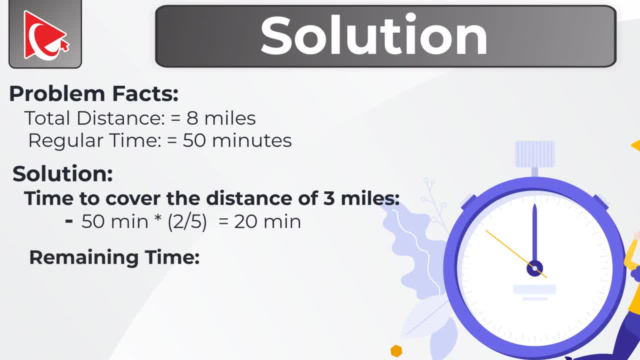 so the remaining time to cover the remaining distance would be 50 minutes minus 20 minutes, which would be 30 minutes, which would be half an hour. Hm. here's how it goes. We need to calculate the remaining distance, for example. 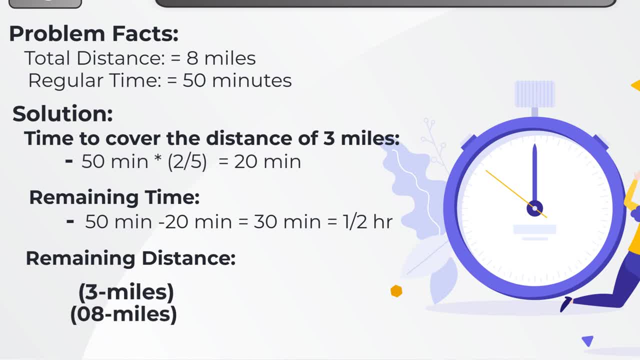 in place of the remaining distance. So she claimed 30 minutes, Since she covered 3 miles and total distance is 8 miles. we won't change for this time. we're only going to calculate 20 minutes. We'll calculate 20 minutes. 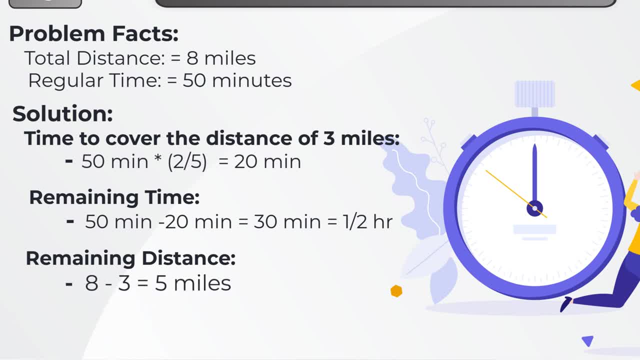 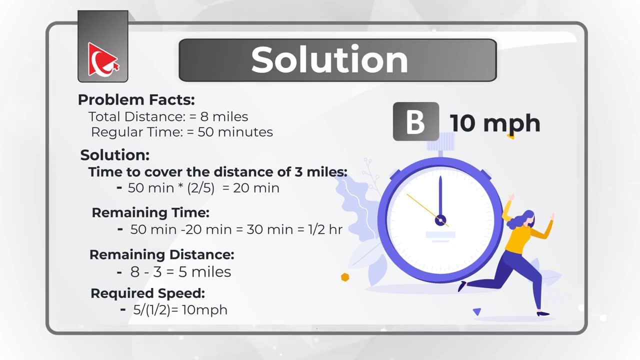 three miles would be equal five miles. ultimately, she would need to cover five miles in half an hour. to determine the speed that you need to go with, we need to divide five by one and a half, and five divided by 0.5 equals 10.. so the correct solution is choice b, 10 miles per hour. were you able to? 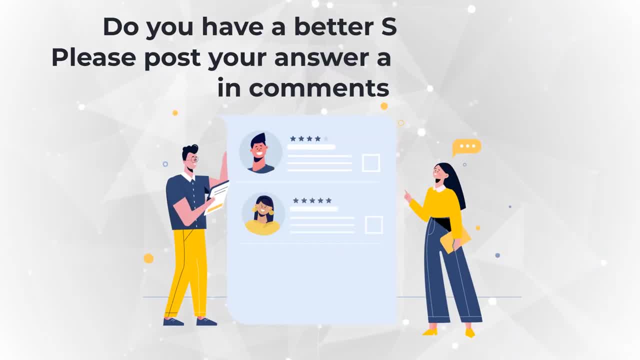 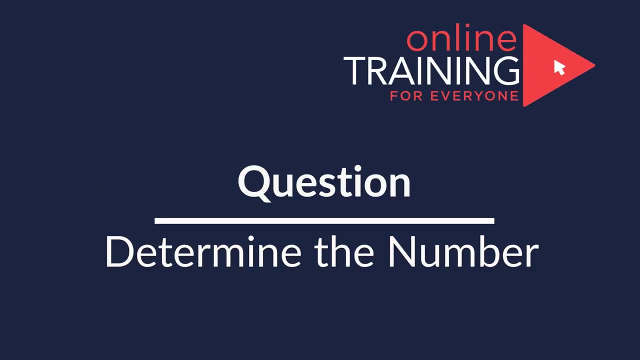 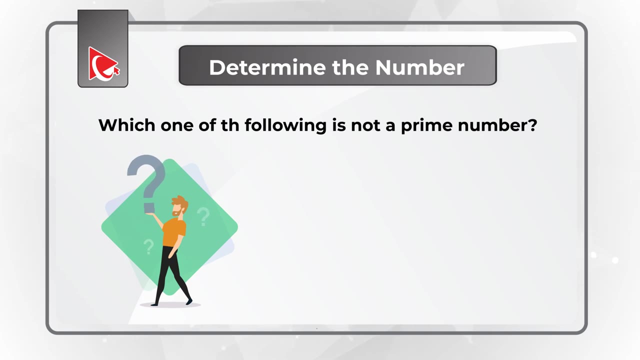 solve it on your own. do you have an alternative solution? please make sure to post your thoughts and feedback in comments. here's an interesting question where you present it with the set of numbers and you need to determine which number is not a prime number. you have four different choices. 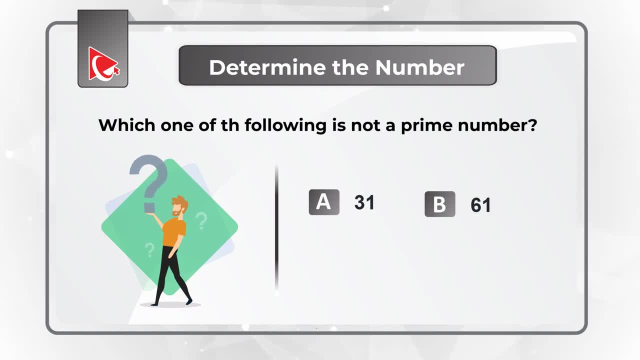 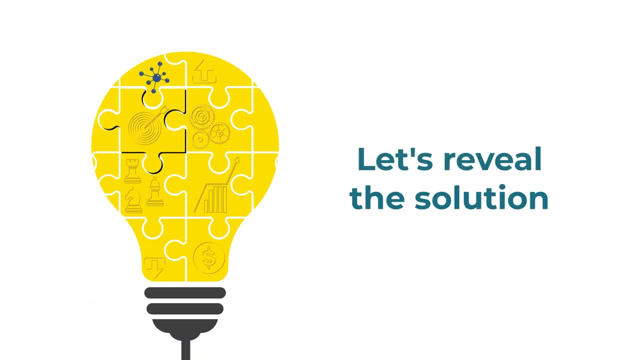 choice a: 31, choice b: 61, choice c: 71 and choice d: 91. give yourself a little bit of time. maybe recall the definition of prime numbers and see if you can come up with the solution. did you solve it? let's move forward and get to the correct solution together. 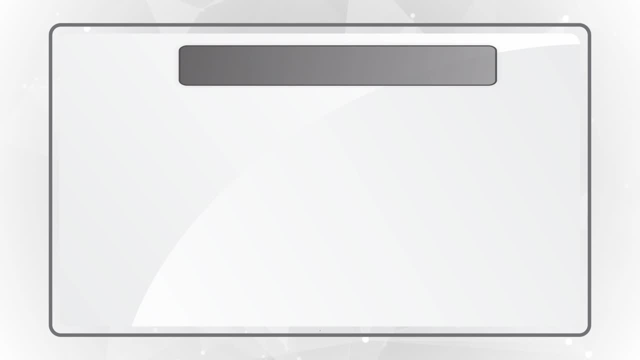 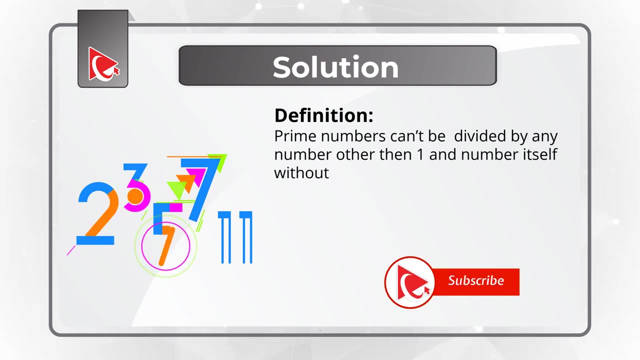 to solve this challenge, let's start with the definition of prime number. prime numbers cannot be divided by any number other than one and number itself without leaving a remainder. some examples of prime numbers would be two, three, five, seven, eleven, and you can continue the chain. the opposite of prime numbers are composite numbers and 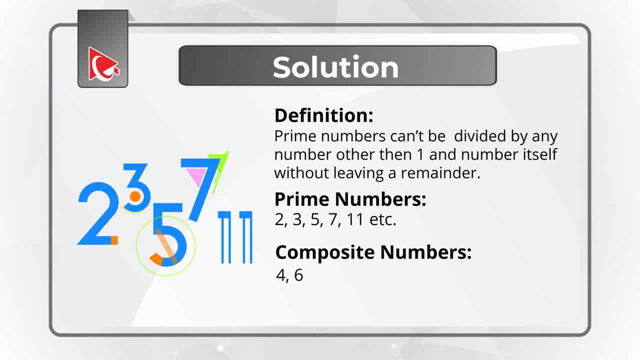 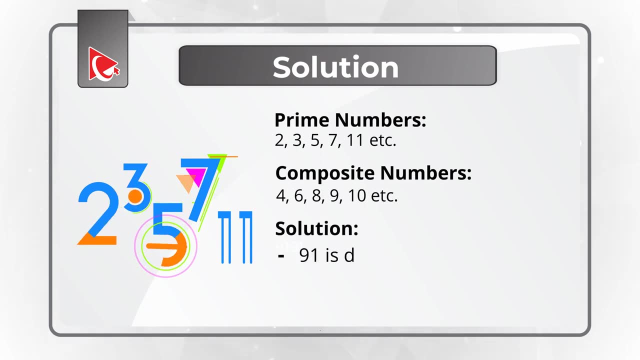 examples of those would be: four could be divided by two, six could be divided by two and three, eight, which could be divided by two and four, nine, ten, and you can continue the sequence. as you might have figured out out of the numbers presented, ninety one can be divisible by seven, so 91 is not. 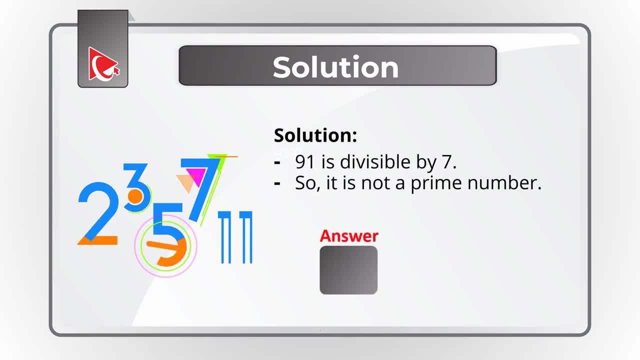 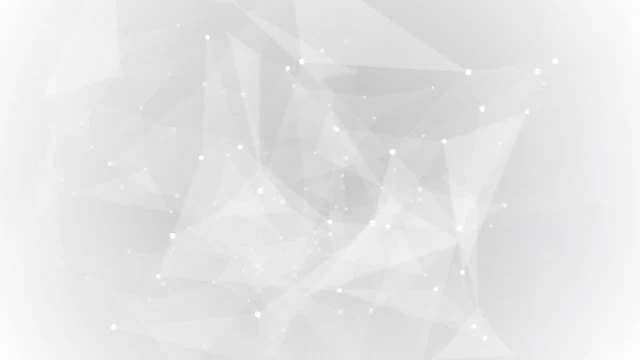 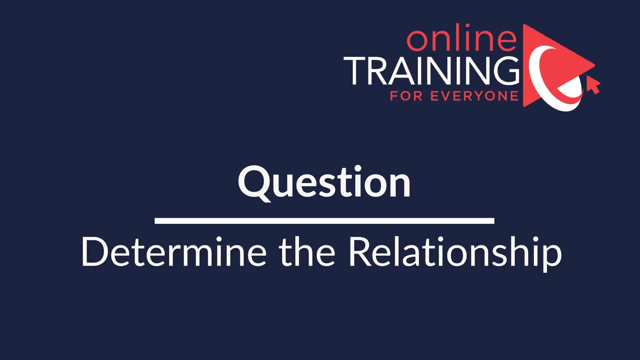 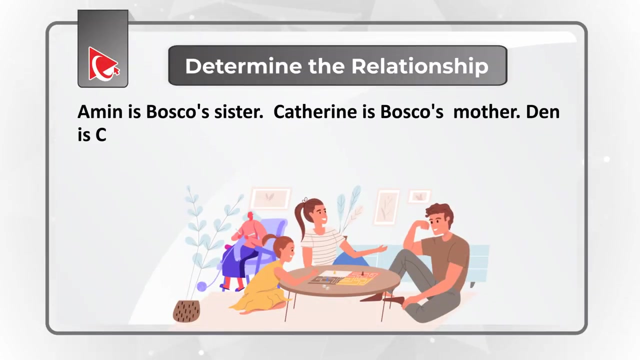 a prime number, which means that the correct solution is choice d, 91.. hopefully you've nailed this question and now know how to answer similar problems on the test. here's an interesting challenge where you need to determine the relationship between family members: amin is baska's sister, catherine is baska's mother, dan. 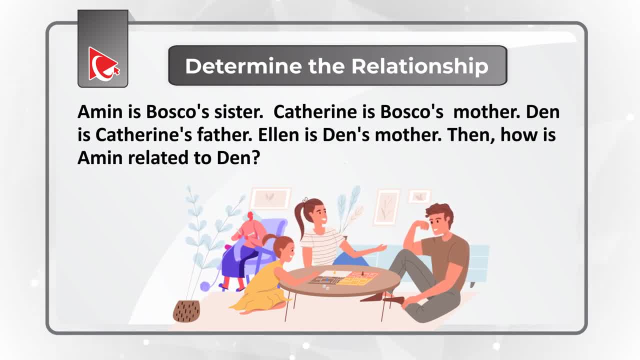 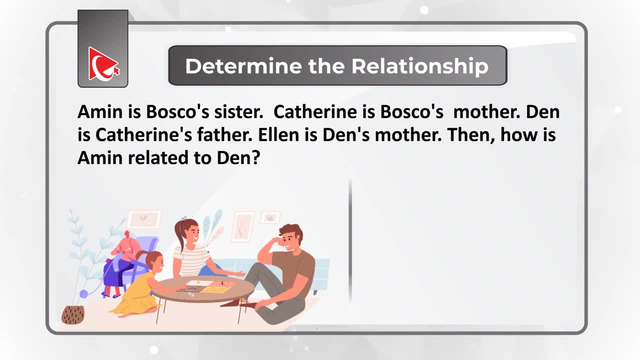 is catherine's father and ellen is dan's mother. you need to determine how amin is related to den and you have four different choices: choice a- grandfather, choice b- grandmother, choice c- daughter and choice d- granddaughter. give yourself a little bit of time to see if 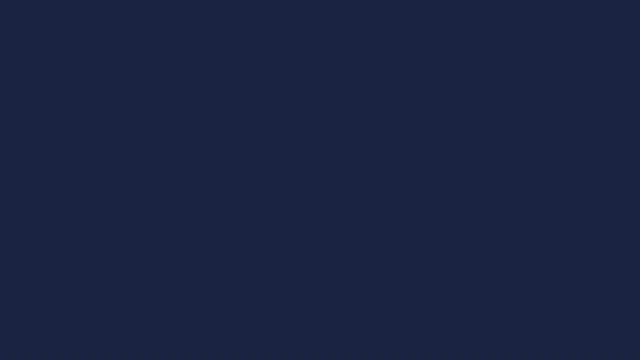 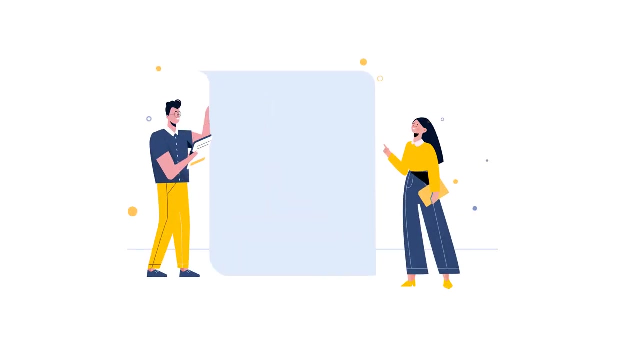 you can navigate in this puzzle and get to the correct solution, ready or not, i am going to move forward, reveal the answer to you, you and explain how I got to the solution And, as usual, if you have a better way to solve it, please make sure to share in comments. 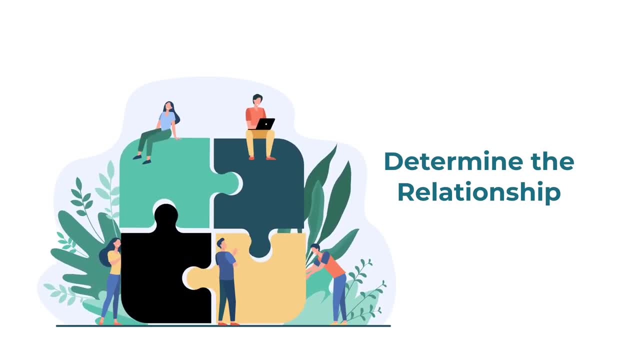 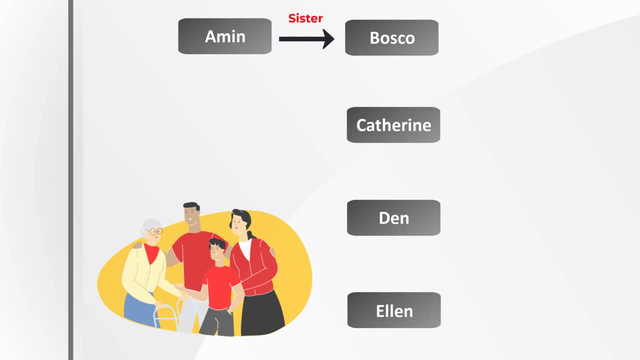 The easiest way to determine this multigenerational relationship in the family is to build a diagram. Let's do it one step at a time. Amin is Basko's sister. Catherine is Basko's mother. Dan is Catherine's father. 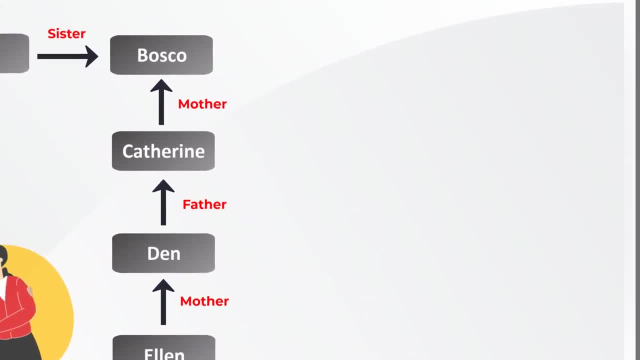 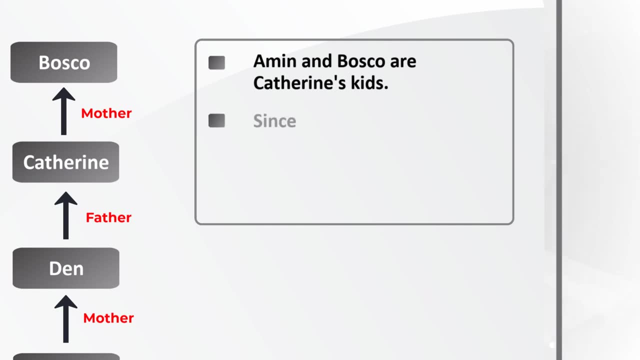 And Ellen is Dan's mother. Now let's look at the conclusions we can draw from this diagram. Amin and Basko are Catherine's children. Since Dan is Catherine's father, Amin and Basko are Dan's grandkids. 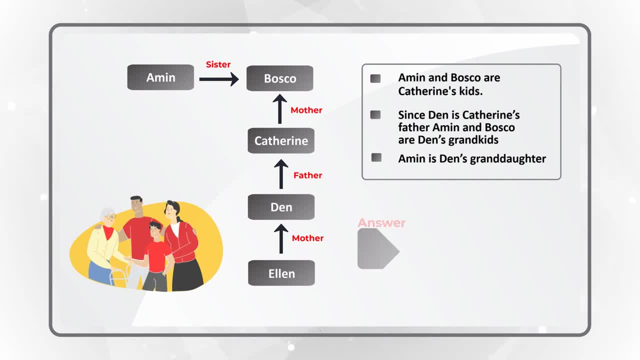 Which means that Amin is Dan's granddaughter. So the correct choice here is choice D- granddaughter. Hopefully you've nailed this question and now know how to diagram and solve similar problems on the test. Here is the frequently used question To test how we solve a multigenerational relationship in the family. we need to know how to solve. 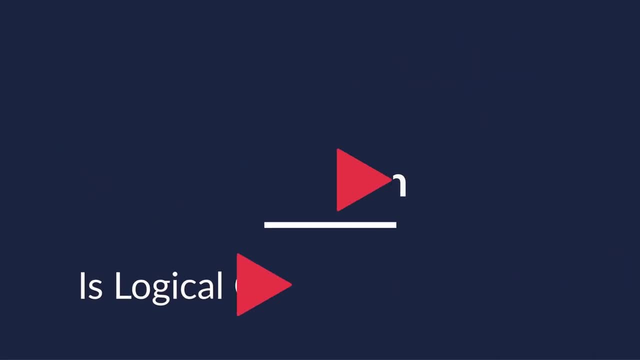 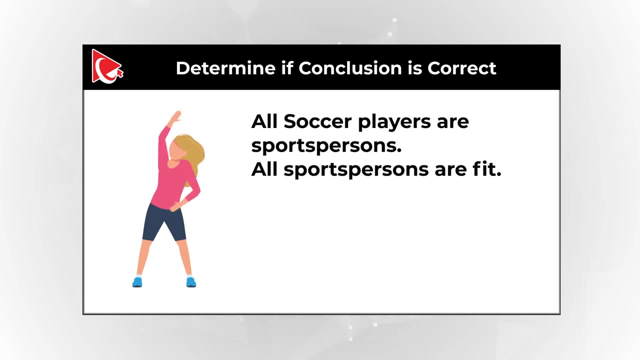 it? How logical are you? You need to determine if the conclusion is correct based on the statements. Let's look at the statement: All soccer players are sportspersons And all sportspersons are fit. Conclusion: Some soccer players are not fit. 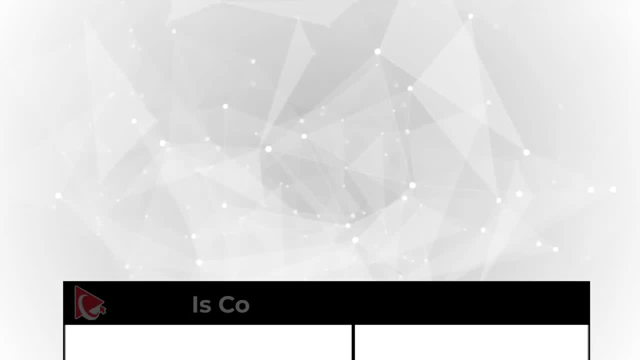 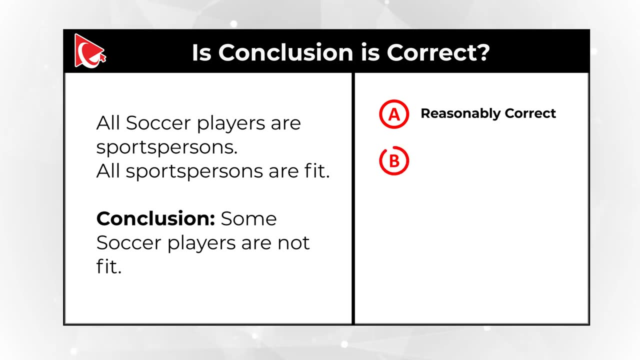 And you need to determine if this particular conclusion is correct. You have four different choices to determine if the conclusion is accurate: Choice A- It's reasonably correct, Choice B- It is correct, Choice C- It is incorrect. And choice D cannot be determined based on the information available. 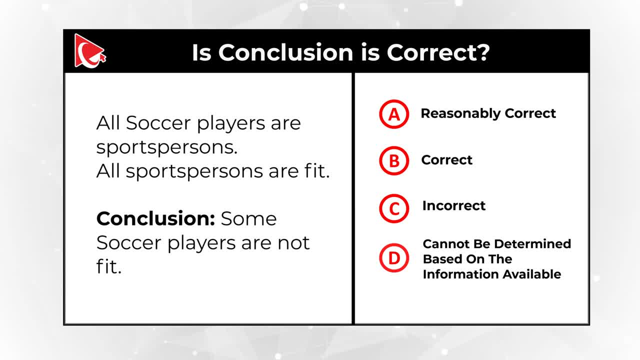 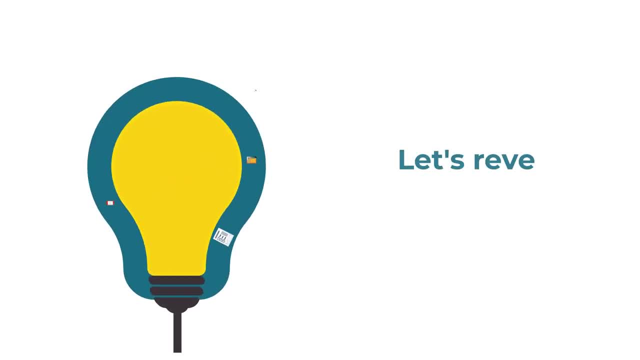 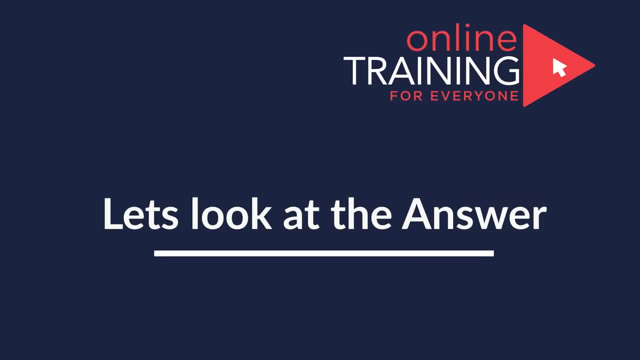 Do you think you know the answer? Give yourself a little bit of time. Maybe pause this video and take another look at the statements and at the question itself. Ready or not? I am going to move forward and reveal the solution. As you might be well aware, in a logical world there is a formula. 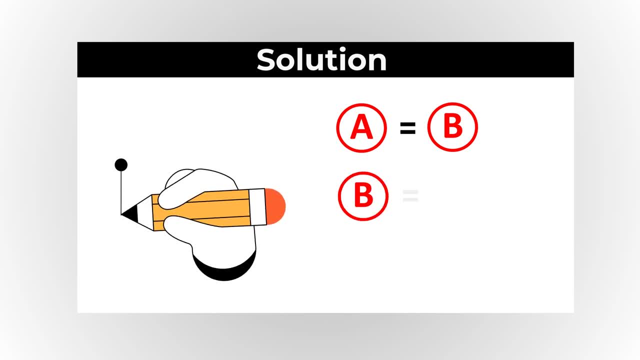 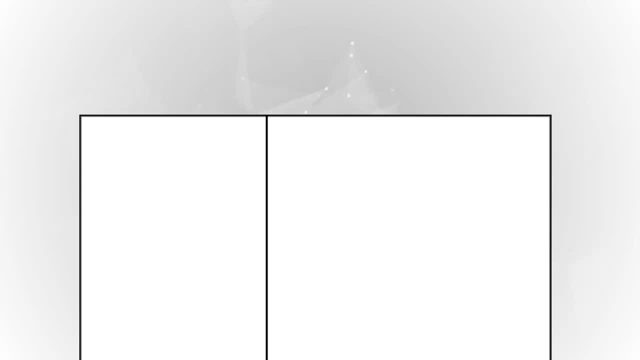 If A equals B, then B equals C, A equals B and B equals C, then you can reasonably conclude that A equals C as well. We can look at our original statements as A, B and C, For example the statement. 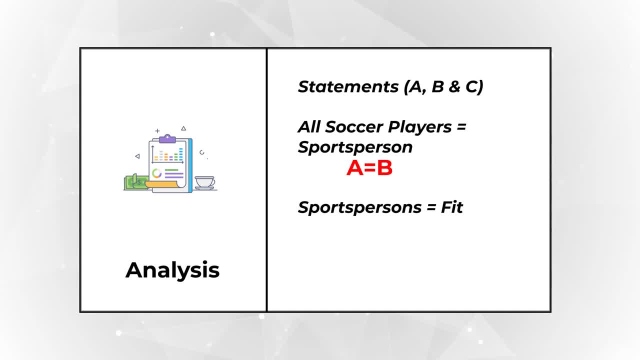 all soccer players are sportspersons could be an equivalent of A equals B, and that all sportspersons are fit could be B equals C. Based on these two statements, we can reasonably say that A equals C, which would mean that all soccer players are fit. 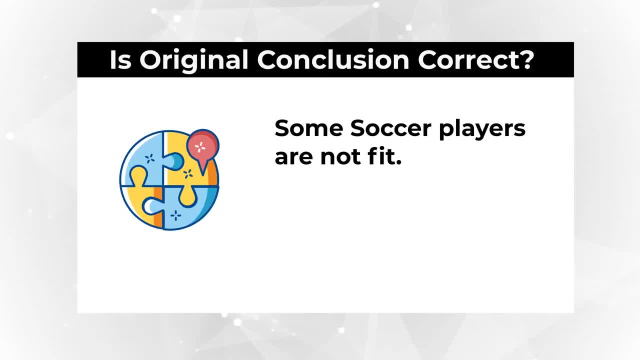 Our question, though, asks us: if some soccer players are not fit, Do you think it is correct Based on the information provided? it is not correct. so the correct choice here is choice C. incorrect because the correct answer, based on the information we have, is: all soccer players are fit. 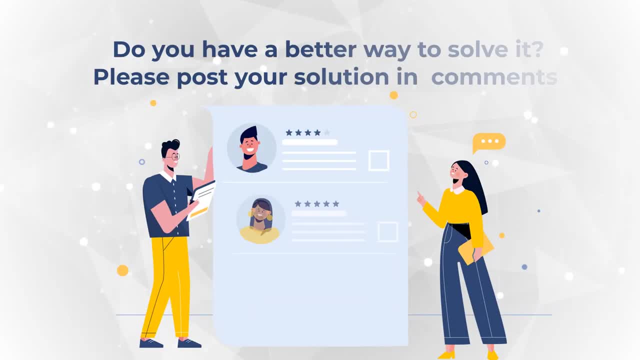 Do you have a better way to solve this question? Please make sure to share in comments. And if you're trying to get ready for the test and need additional questions to practice, please make sure to check out additional materials in the description section of this video. 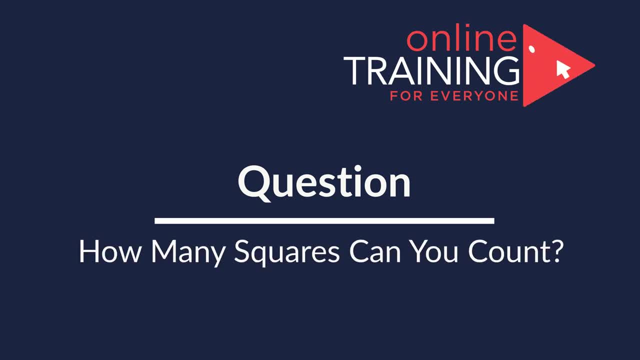 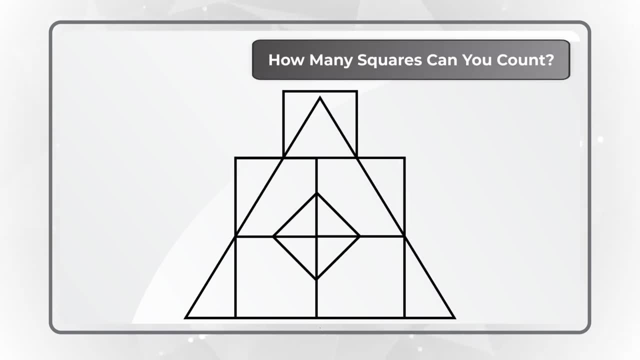 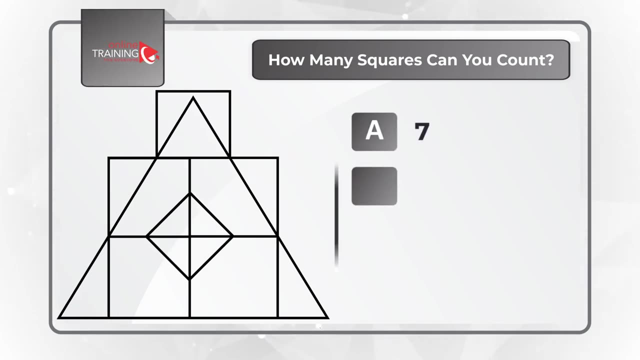 There is something fascinating about the questions where you need to count the number of squares. Let's look at the picture presented on the screen. How many squares can you count? You have four different choices. Do you see 7 squares, or 8 squares, or 9, or 12 squares? 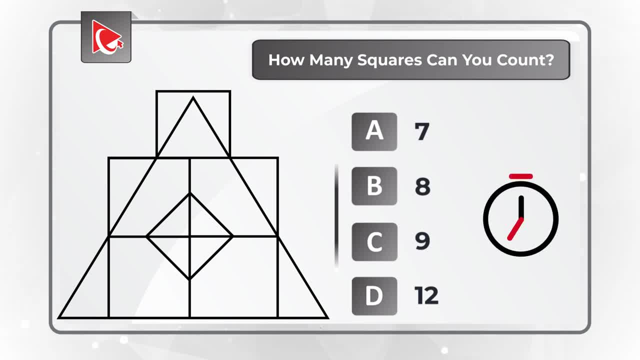 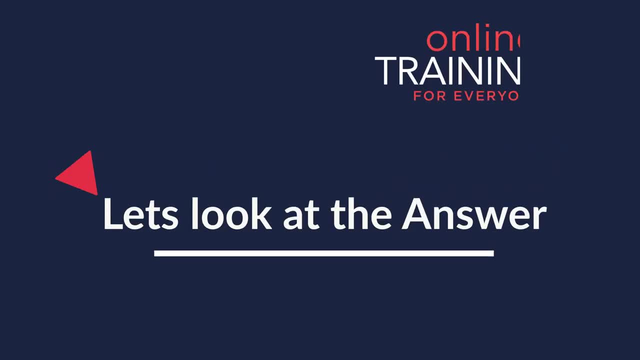 Give yourself a little bit of time to think about it And, if you have time, maybe pause this video to see if you can come up with the solution. I counted 7 squares, so my answer is choice A. Let me show them all to you. 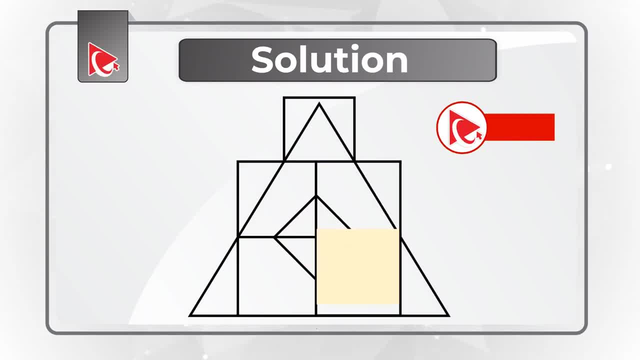 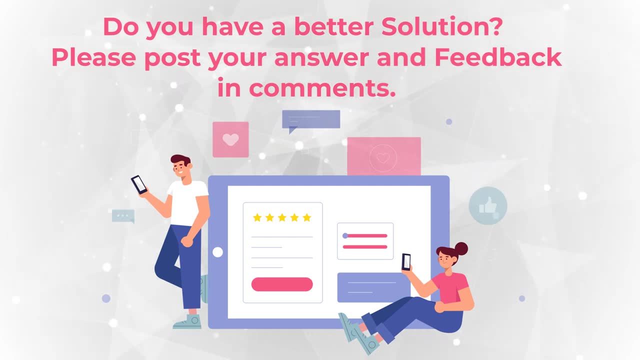 1,, 2,, 3,, 4,, 5,, 6, and 7.. Do you have a different number? Please make sure to post your solution in comments, And if you need more questions like this, please make sure to check out description for additional resources. 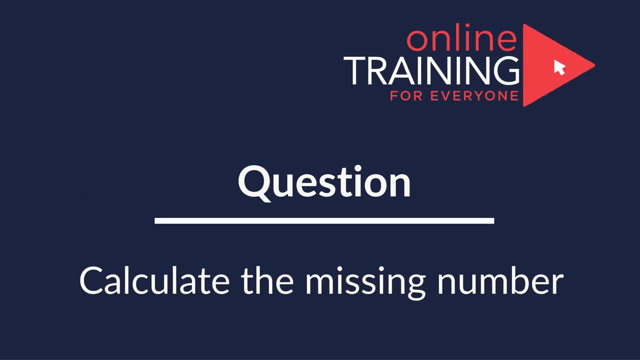 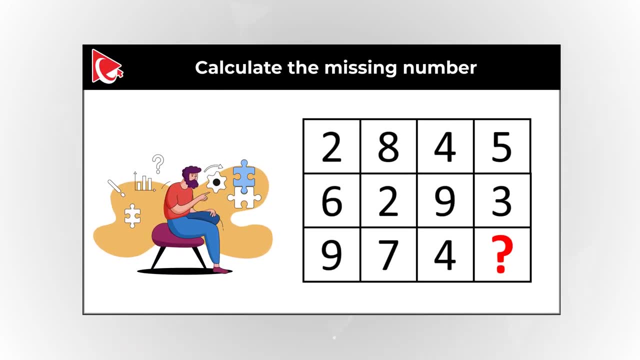 Here is one of my favorite questions, which validates if you can think out of the box. You are presented with the rectangle which contains three rows. First row has numbers 2,, 8,, 4, and 5.. Second row has numbers 6,, 2,, 9, and 3.. 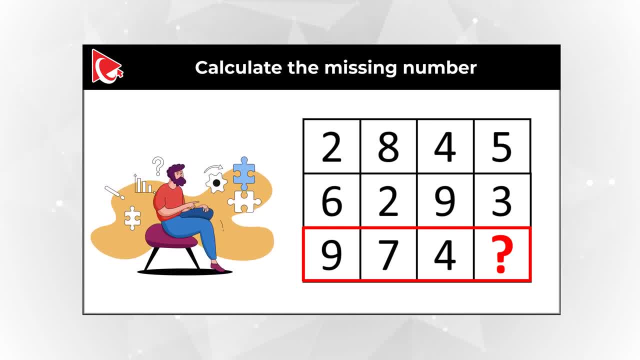 And the last third row has numbers 6,, 2,, 9, and 3.. And the last third row has numbers 9,, 7,, 4, and then the fourth number is missing. Can you calculate it? 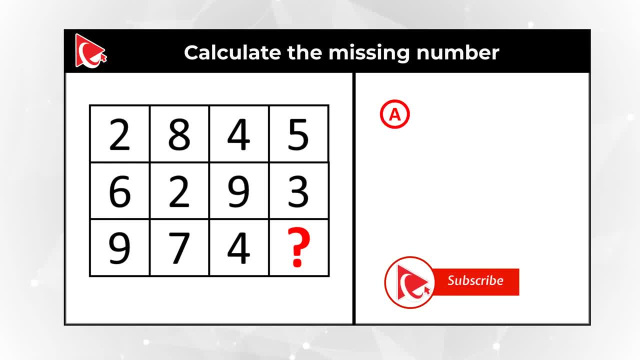 You are presented with four different choices: Choice A: 7. Choice B: 8.. Choice C: 9. And then choice D, 12. Give yourself a little bit of time to see if you can do the calculations. Maybe pause this video to see if you can come up with the solution. 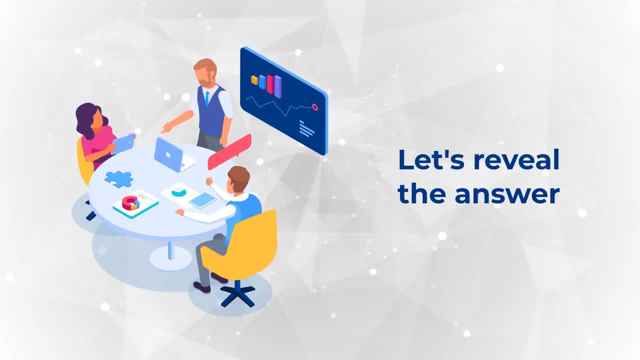 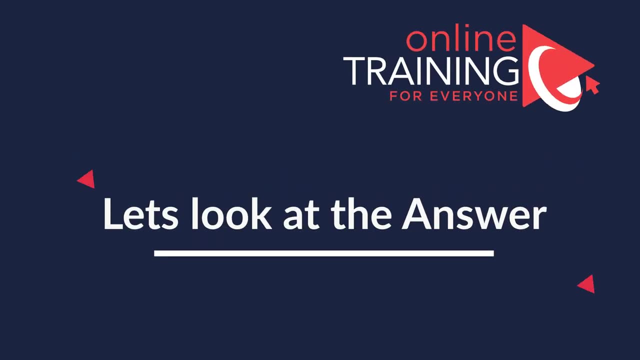 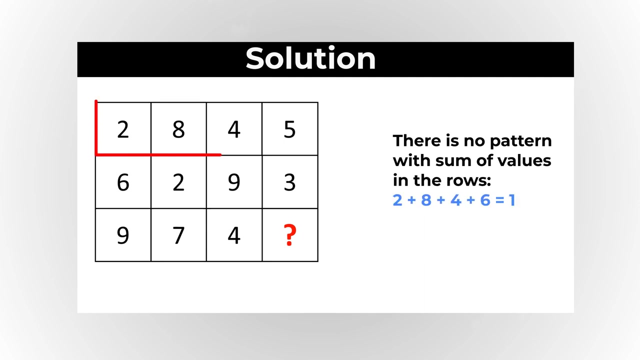 Are you ready? Let's move forward and get to the correct solution together, As usual. my advice to you: look for patterns. Let's first check the patterns in the rows. Let's sum up the values in the row: 2 plus 8 plus 4 plus 5 equals 19.. 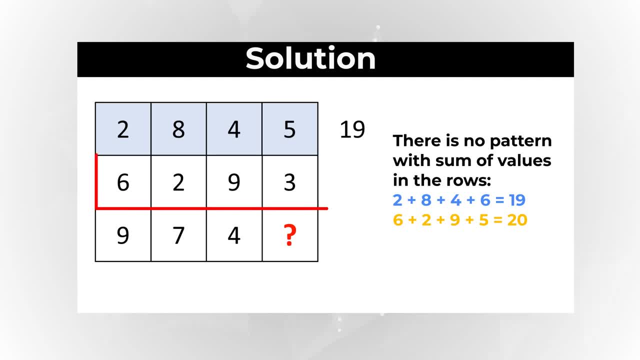 Second row: 6 plus 2 plus 9 plus 3 equals 20.. Looks like there is no pattern. I don't see any pattern, do you? Let's check the columns. The first column has rows. It has values 2 plus 6 plus 9.. 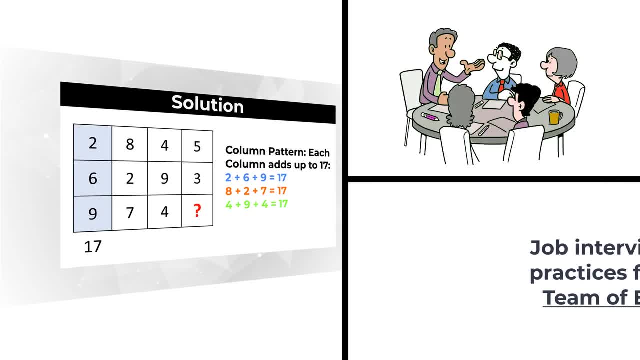 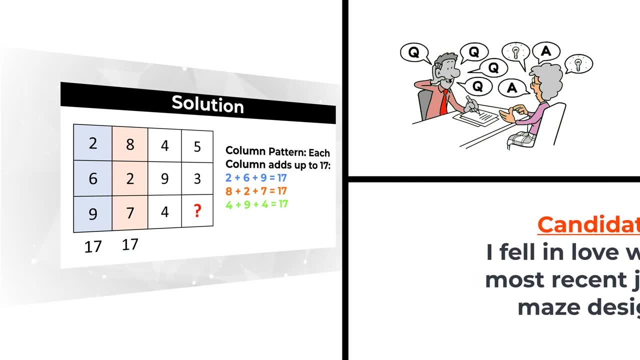 Some of those equals 17.. Let's look at the second column: 8 plus 2 plus 7 also equals 17.. I think we are getting somewhere. And then the third column is 4 plus 9 plus 4 also equals 17.. 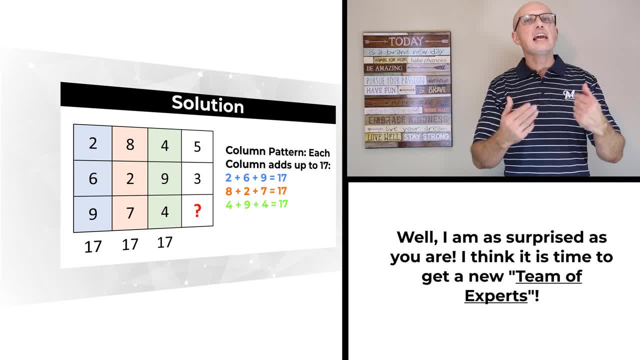 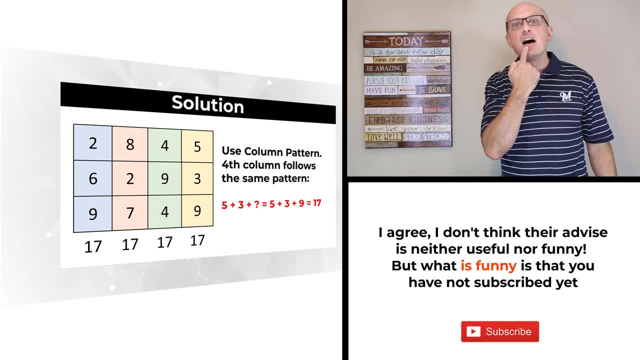 Based on this information, we can calculate the missing value. 5 plus 3 plus question mark would be equal. 5 plus 3 plus 9 also equals to 17. So the correct choice here is choice C 9.. Hopefully you've nailed this question and now know what to look for on the similar problems. 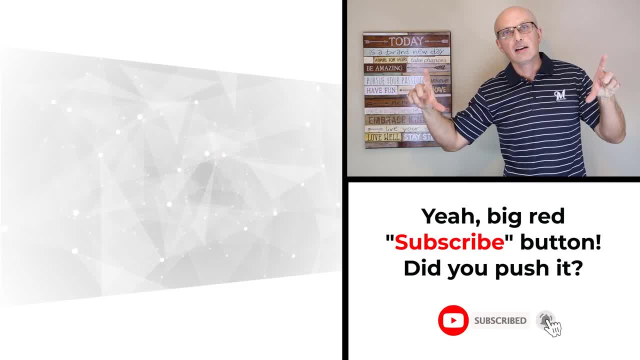 on the test. Here is a tricky problem that you might find challenging to solve. You are presented with the pyramid. Top of the pyramid starts with the missing number that you need to calculate If you go down. second row contains numbers 29 and 34.. Next row contains numbers 11,, 12,, 13,, 14,, 15,, 16,, 17,, 18,, 19,, 20,, 21,, 22,, 23,, 24,, 25,, 26,. 26,, 27,, 28,, 29,, 30,, 31,, 32,, 33,, 34,, 35,, 36,, 37,, 38,, 38,, 39,, 40,, 41,, 42,, 42,, 43,, 44,. 45,, 45,, 45,, 46,, 47,, 48,, 49,, 41,, 42,, 45,, 45,, 46,, 47,, 49,, 41,, 42,, 45,, 45,, 46,. 50,, 65,, 60,, 71,, 42,, 44,, 45,, 85,, 74,, 66,, 87,, 88,, 89,, 90,, 91,, 92,, 93,, 92,, 93,. 94,, 92,, 93,, 92,, 94,, 99,, 95,, 100,, 92,, 93,, 94,, 91,, 92,, 94, 1, 2, 1, 2, 2, 2, 1, 2, 1, 2,. 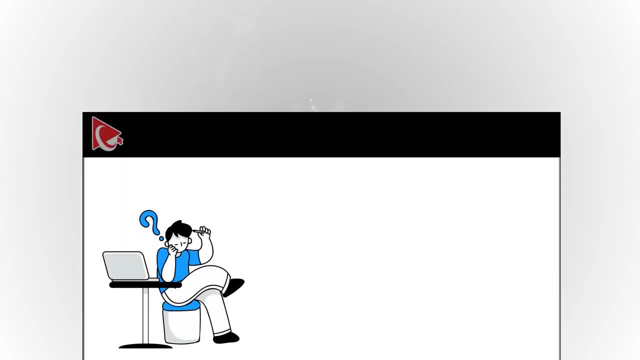 2. The right-hand side of the pyramid starts with the missing number that you need to calculate. Here is a tricky problem that you might find challenging to solve. You are presented with the pyramid. Top of the pyramid starts with the missing number that you need to calculate. 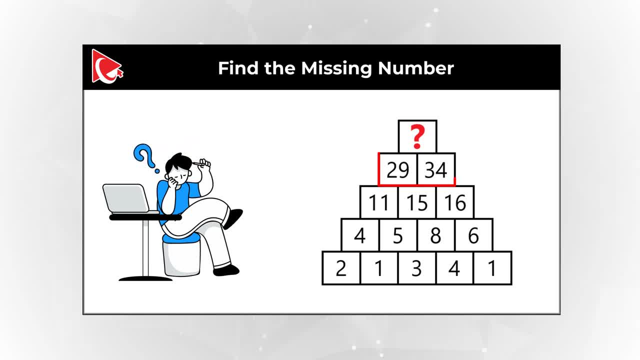 If you go down, second row contains numbers 29 and 34.. Next row contains numbers 11,, 15, 16.. Following row has numbers 4,, 5,, 8, and 6.. And then the last row has numbers 2 and 7.. 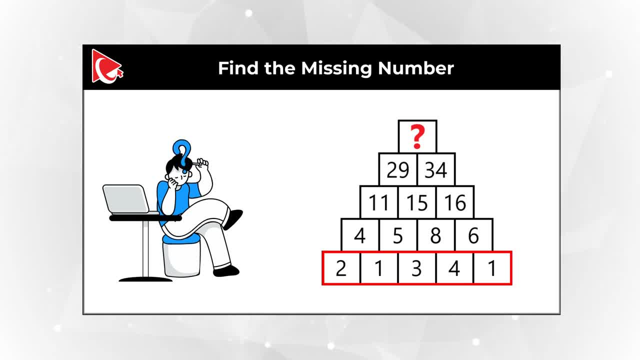 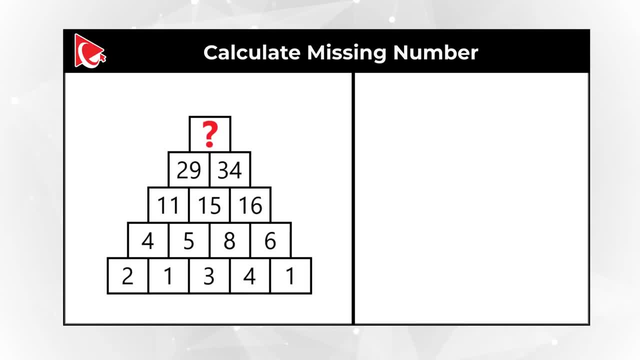 4,, 5,, 8, and 6.. 2,, 1,, 3,, 4 and 1.. You need to calculate the missing number, which is in the top row, and you have four different choices: Choice A- 59.. Choice B- 63.. Choice C- 67 and then choice D- 73.. Give yourself. 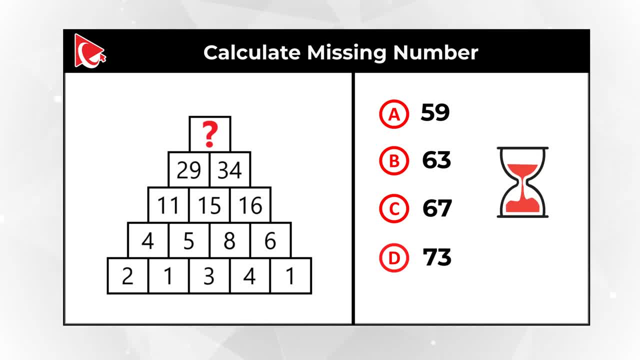 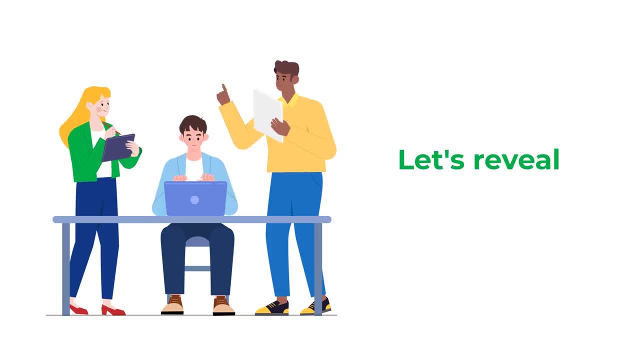 a little bit of time- maybe 10 to 15 seconds, maybe a little bit longer- to see if you can answer this question. Did you solve it? Was it hard for you? Let's move forward and I'll share with you my solution, But obviously, if you have a better way to solve it, please make sure to post it in. 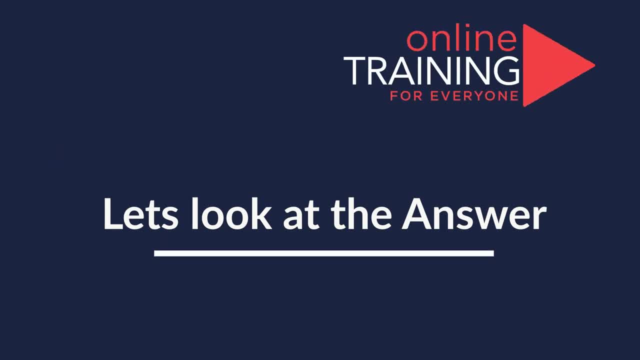 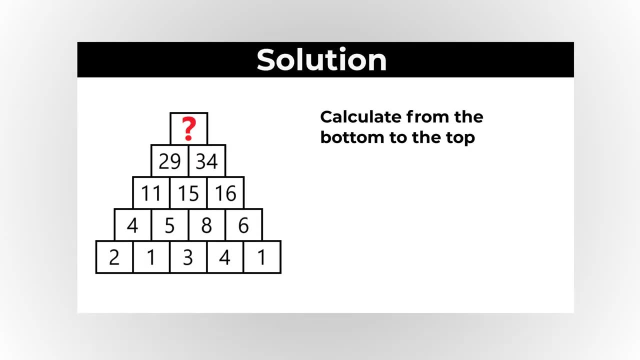 comments. Tricky problem, don't you think so? But the solution to this challenge is really simple. To calculate it correctly, you need to move from the bottom to the top, and if you look closely at the pyramid, you will notice that the higher row is calculated from the bottom to the top. 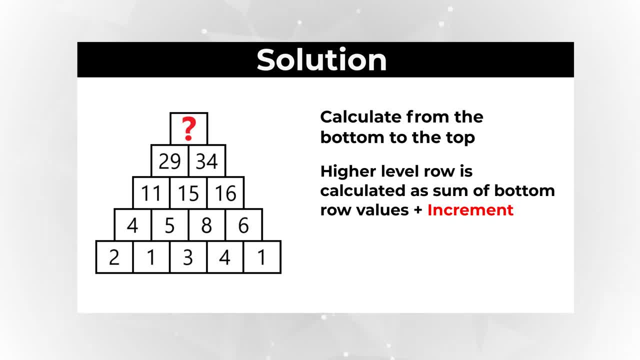 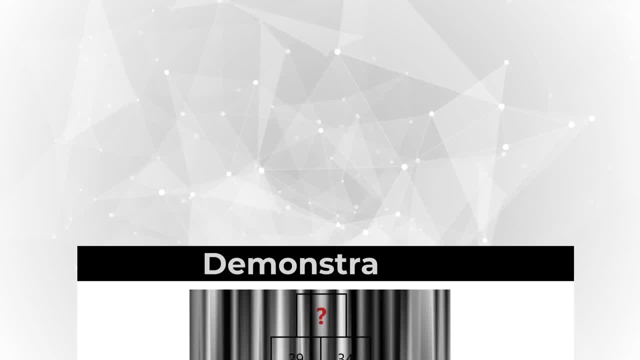 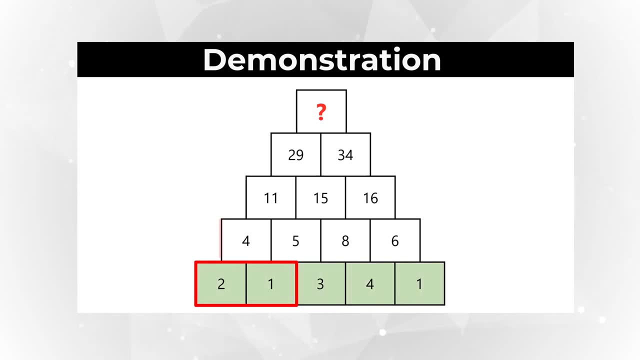 The bottom row is calculated as the sum of bottom values plus the increment. An increment also increases with each row by one. Let me demonstrate. If we look at the numbers in the bottom left corner of the pyramid, you see numbers 2 and 1.. Sum of 2 and 1 is 3, but then we add the value of the. 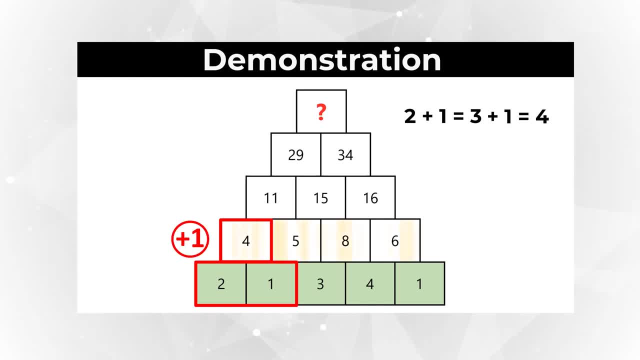 increment, which is 1, and the calculated value is 4.. Let's continue with the sequence. Next set of numbers is 4 and 5.. 4 plus 5 is 9, and then we need to add the value of the increment, which also. 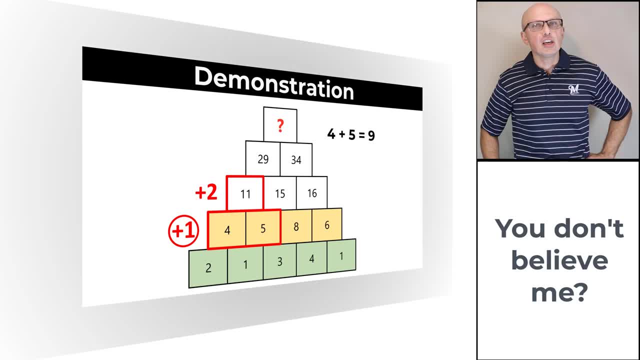 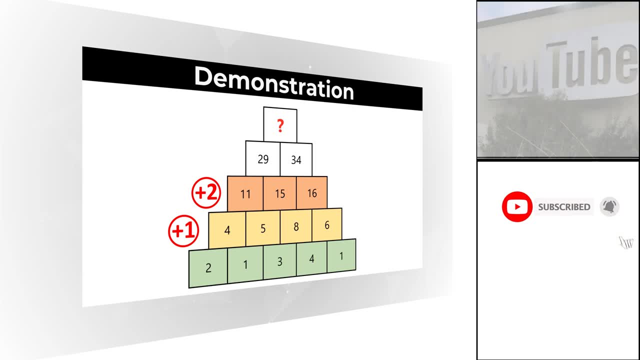 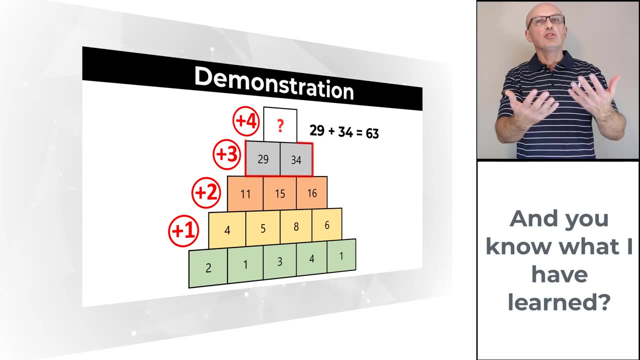 increased by one. So now, instead of being plus one, the increment is plus 2.. 4 plus 5 plus 2 equals 11.. Based on this information, the missing value can be calculated as 29 plus 34 plus the value of the increment, which would be plus four, which equals 63 plus 4 plus 4.. 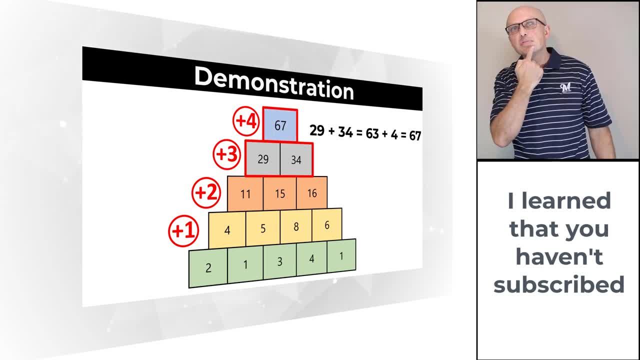 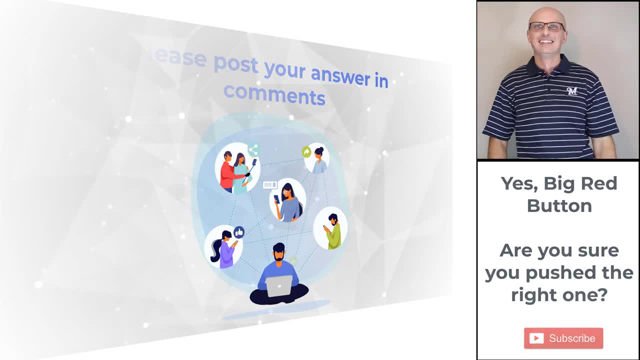 which equals to 67. So the correct choice here is choice C, 67.. Hopefully you've nailed this question on your own and now know how to answer similar problems on the test. Here's an amazing question which tests your imagination and spatial thinking. 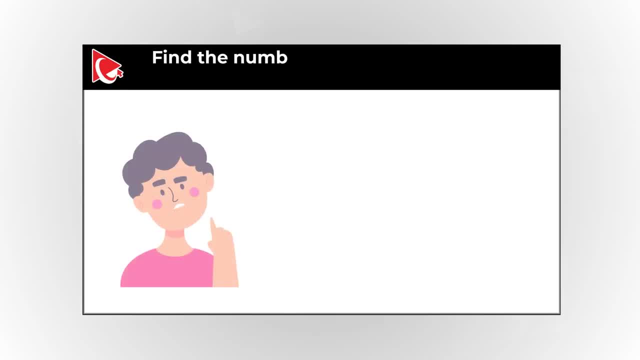 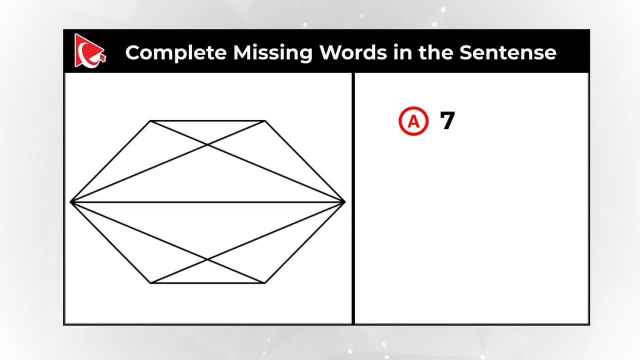 You need to determine how many triangles are shown in this figure. Take a close look and select one out of four different choices: Choice A, 7., Choice B, 10., Choice C, 12. And choice D, 17.. 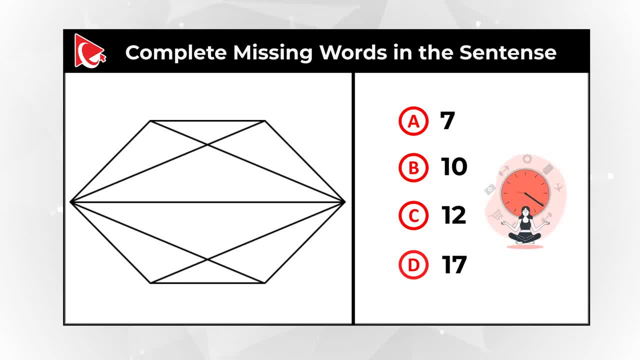 Do you know the answer? Give yourself a little bit of time and use as much of your imagination as possible. Maybe pause this video and give yourself 20 to 30 seconds to determine the answer. Ready or not? I am going to move forward and reveal the solution to you. 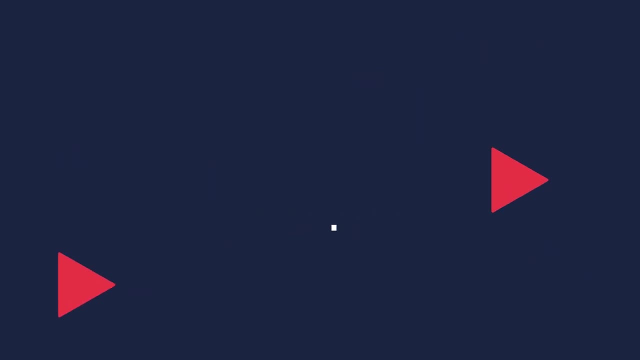 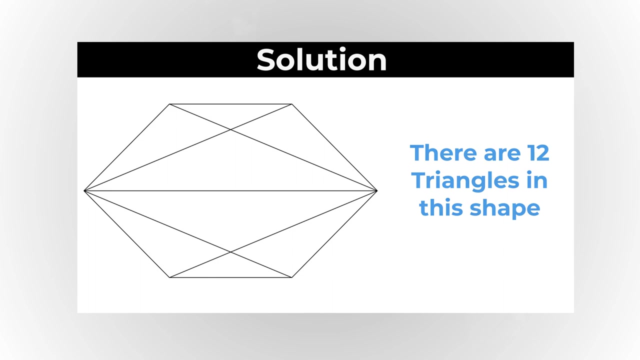 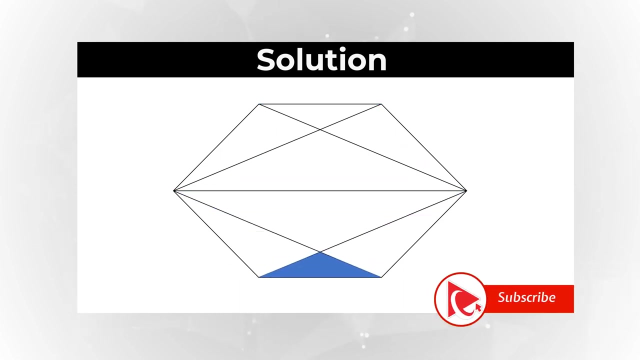 At least the solution I found, And obviously if you have a different solution, please make sure to share it. I couldn't believe it, but I counted 12 triangles here on the picture. Let me show them all to you: 1,, 2,, 3,, 4,, 5,, 6,, 7,, 8,, 9,, 10,, 11, and 12.. 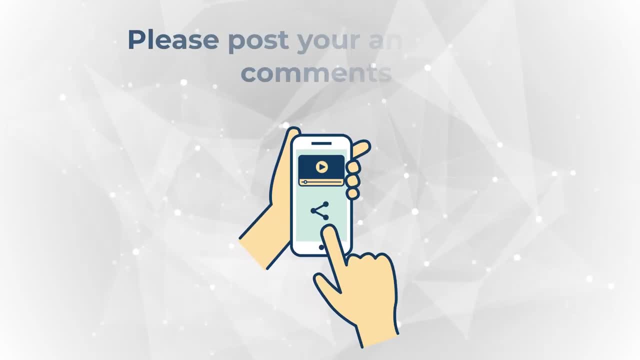 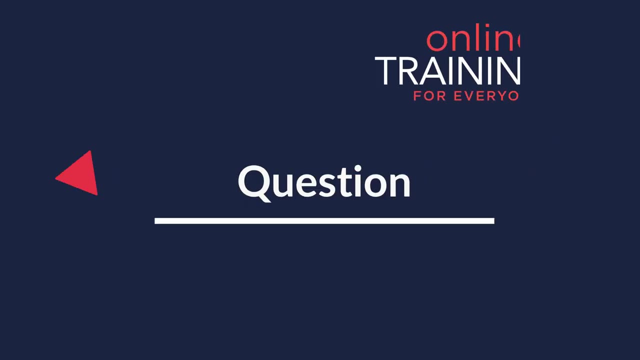 Did you count a different number? Please make sure to share in comments. And also please share. how easy was it for you to guess the answer. If you want to solve it, I'd like to share with you a very interesting question where you need to determine the letter of the alphabet. 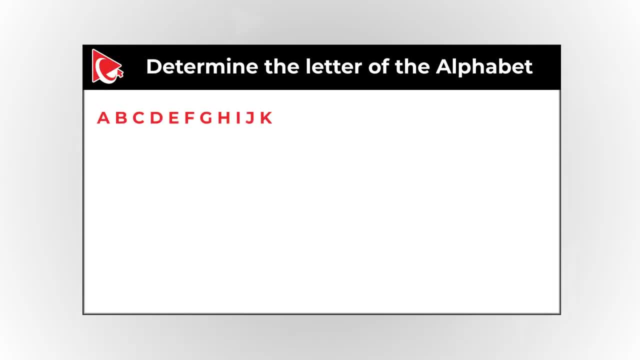 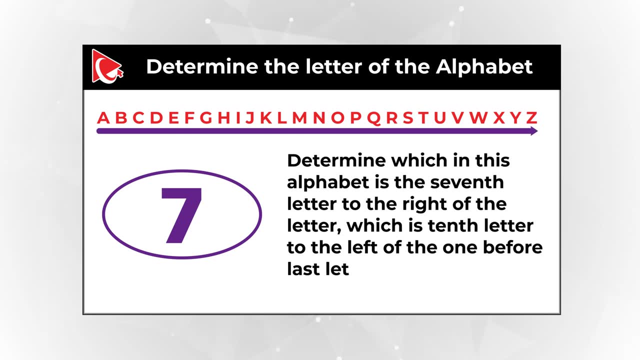 You're presented with 26 letters of English alphabet And you need to determine which letter in this alphabet is the 7th letter to the right of the letter which is 10th letter to the left of the one before last letter of the alphabet. 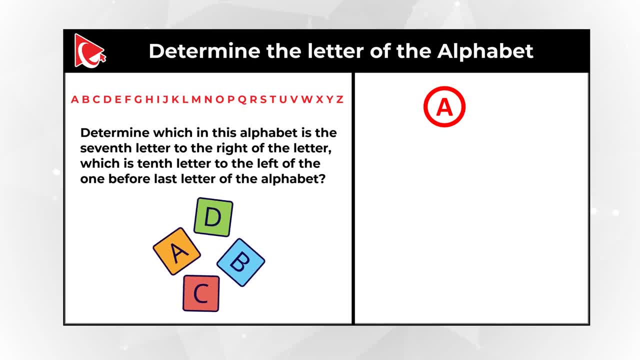 You have four different choices: Choice A- letter X. Choice B- letter W, Choice C- letter V, And choice D- letter O. Can you determine the answer? Give yourself a little bit of time. Maybe pause this video for 10 to 15 seconds. 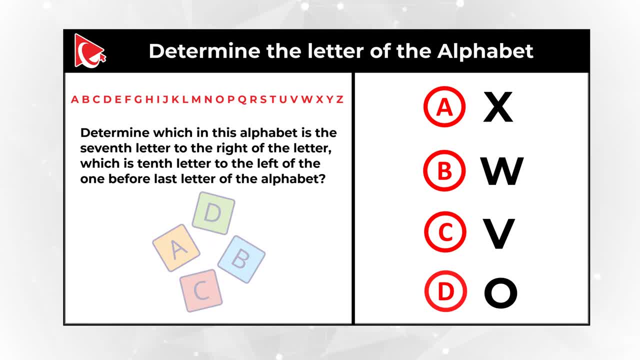 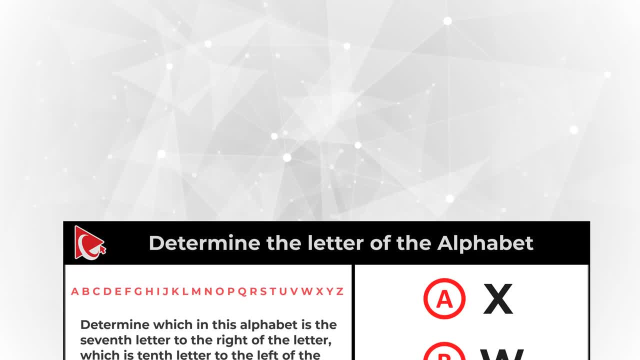 to see if you can come up with the solution. Ready or not, let's move forward and get to the correct solution together. As you might be well aware, there are two ways to solve this problem. The first is to find the right answer. 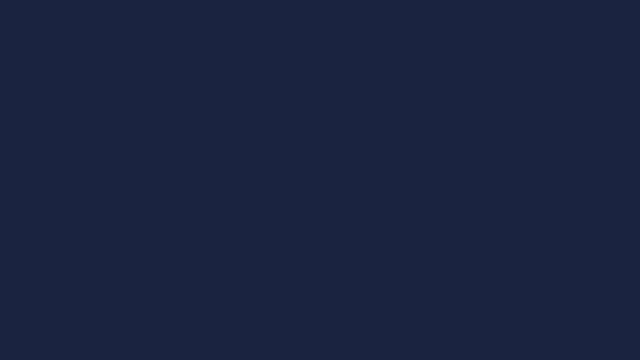 The second is to find the right answer. The third is to find the right answer. The fourth is to find the right answer. In English alphabet there are 26 letters, And the letter one before last is letter Y, 10th letter to the left of the letter Y. 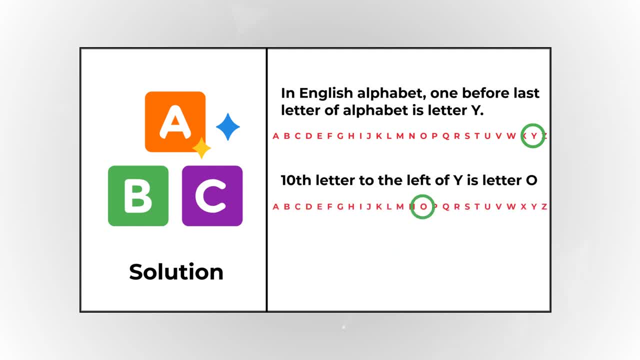 would be letter O. Let me demonstrate it to you. If I am currently at the letter Y, let's count 10 letters to the left of the letter Y. It would be 1, 2, 3, 4, 5, 6, 7. 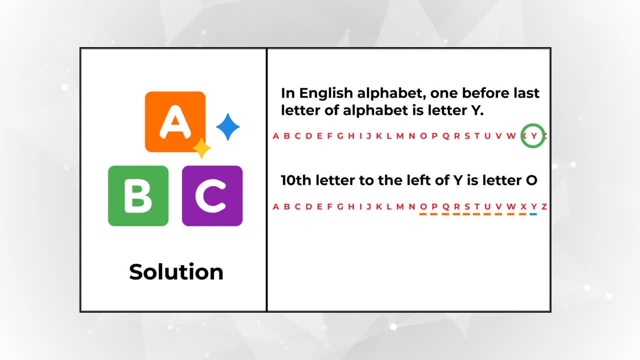 8, 9, 10. You see, I ended up on the letter O. Now we need to determine 7th letter to the right of the letter O. Let's do the math: 1, 2, 3, 4, 5, 6. 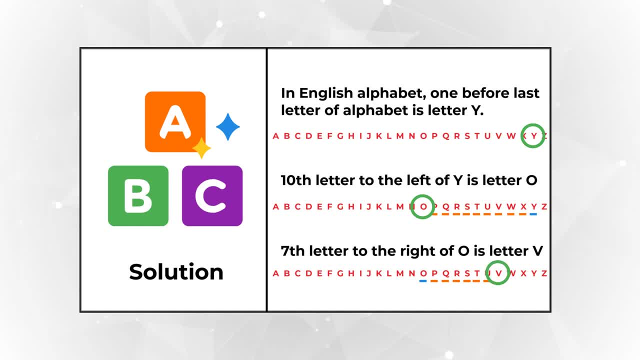 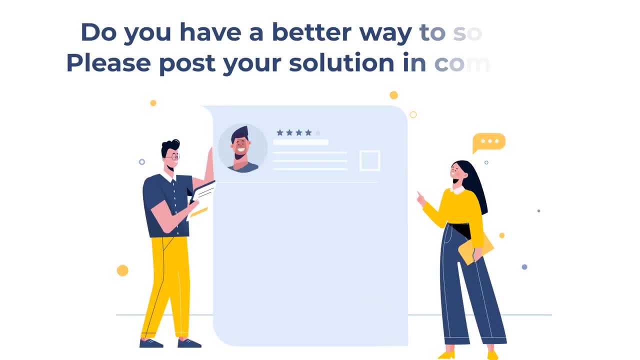 7. As you can see, this is the letter V, So the correct choice here is choice C, letter V. Hopefully you've nailed this question and now know how to answer similar problems on the test, One of the most frequent questions I get. 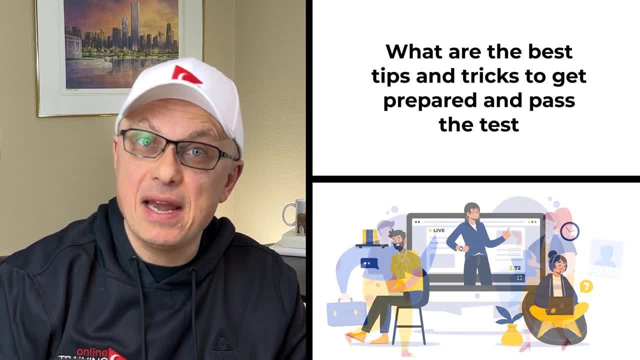 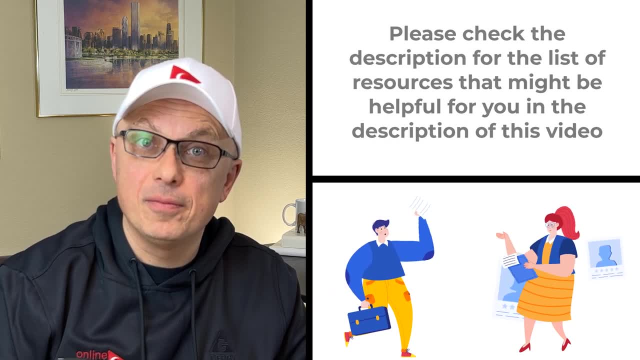 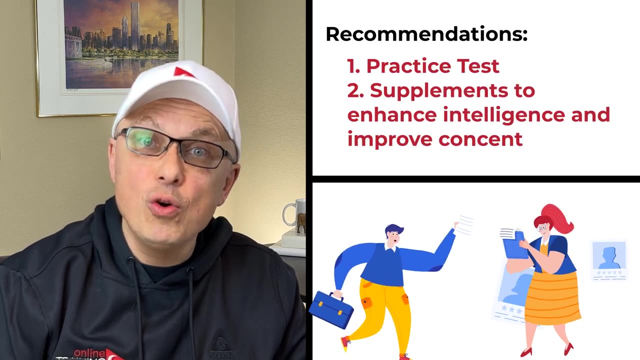 is to provide the best techniques to get prepared and pass the test. We put together a list of resources that might be helpful for you in the description section of this video. Obviously, taking sample tests and reviewing questions and answers is a must, But some less-known ways to improve. 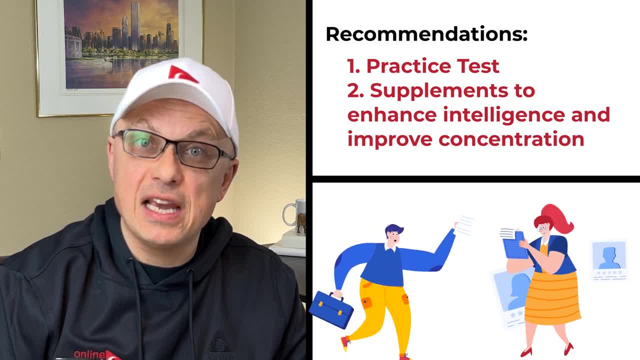 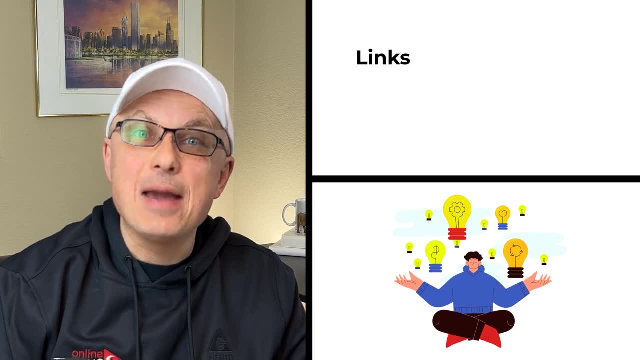 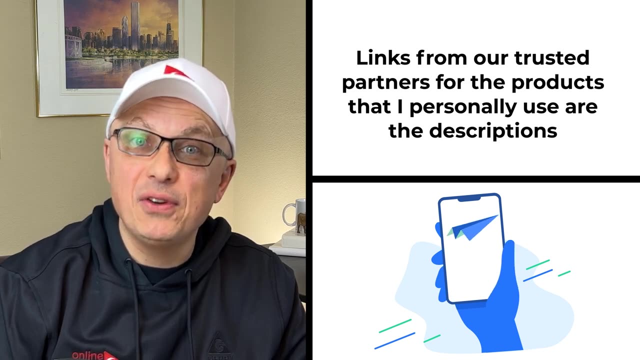 might be to take dietary supplements, sign up for free trials with educational training vendors and even use special supplements to improve your brain function and concentration. I put links to our trusted partners for the products I use in the description section of this video. Some links might be affiliate. 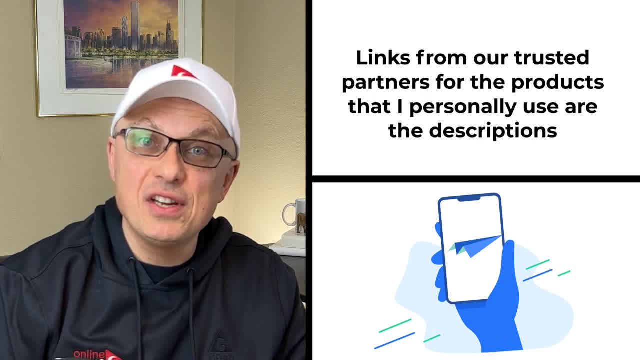 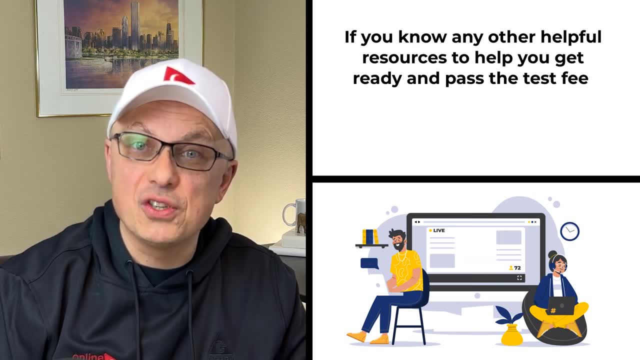 which means that I will get paid a small fee without increasing costs to you. Make sure to check them out. And one request for you: If you know any other helpful resource to help you get ready and pass the test, feel free to share it in comments. 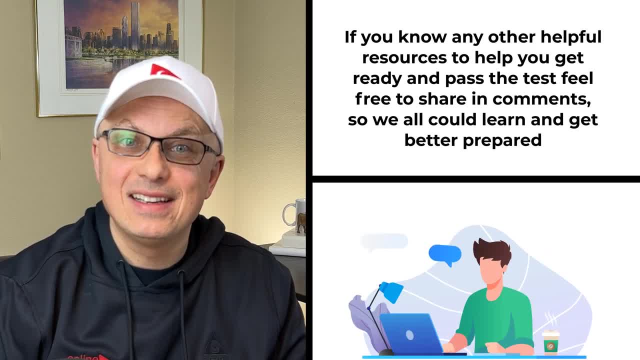 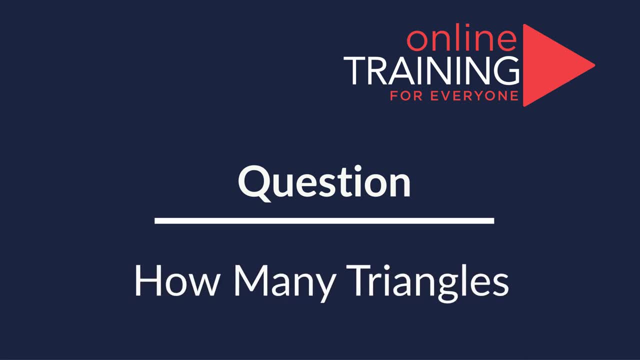 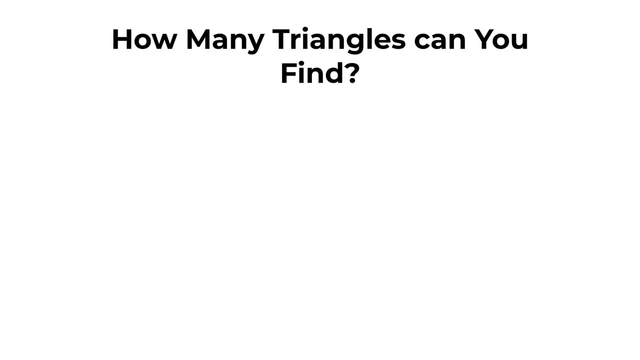 so we could all learn and get better prepared. And now let's continue and get you ready for the test. This particular question was just recently introduced in the test and I would need your help to determine if I answered it correctly. You are presented with the very unusual shape. 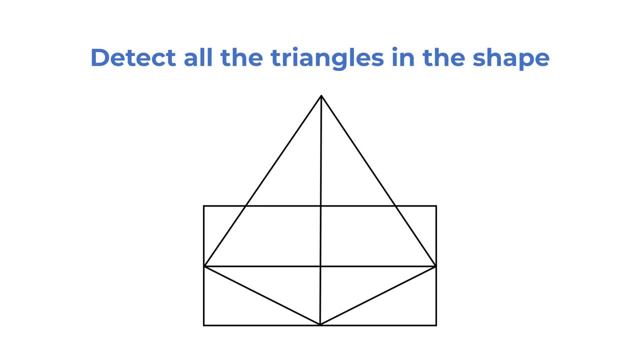 and you need to detect all the triangles that are part of this shape. You have four possible choices: Choice A, 11., Choice B, 13., Choice C, 15. And Choice D, 17.. Do you see the answer? 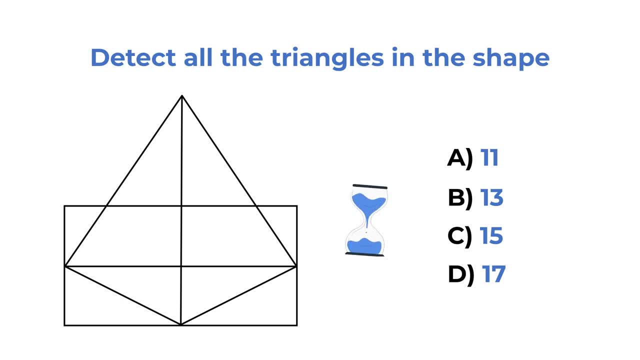 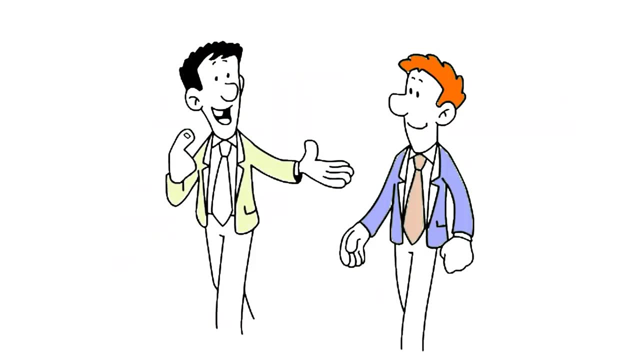 Consider giving yourself a little bit of time, maybe 10 to 20 seconds, to see if you can count all the triangles. Ready or not. I am going to move forward and show you how many triangles did I discover? Tricky question, don't you think so? 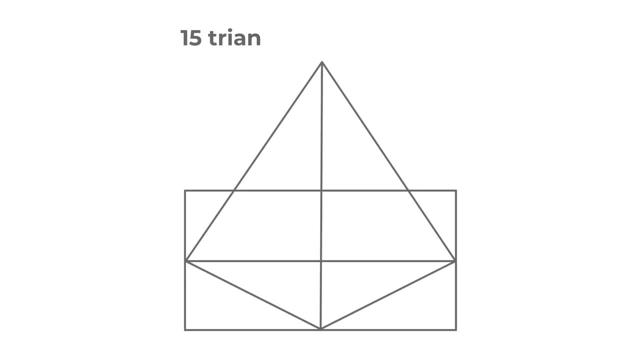 But I was very surprised when I counted 15 triangles in this shape. Let me go over and show all of them to you. Here is the first one, Second, third, fourth, fifth, sixth, seventh, eighth, ninth, tenth. 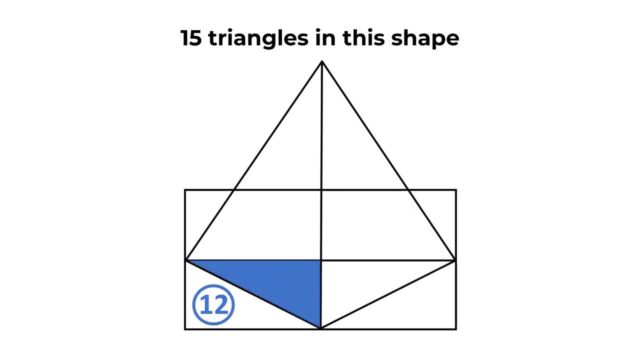 eleventh, twelfth, thirteenth, fourteenth and fifteenth. Do you see any additional ones? Please make sure to pause them in the comment section of this video And, if you are getting ready for the assessment test, please make sure to check out the description. 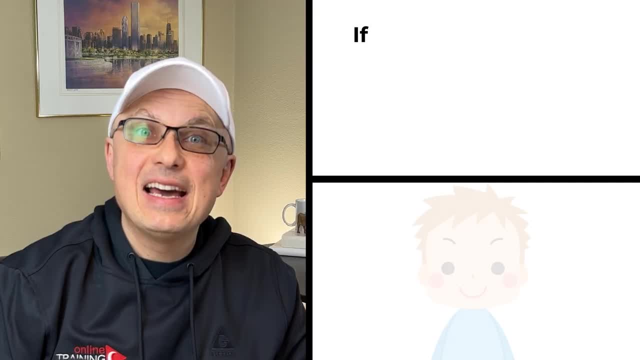 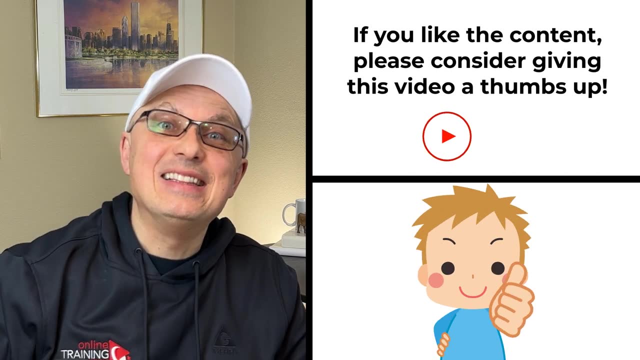 for the link to the e-book that will help you to get ready. Can I ask you to do me a favor? If you like this content, can you please give this video a big thumbs up? This tells us that you need more content like this. 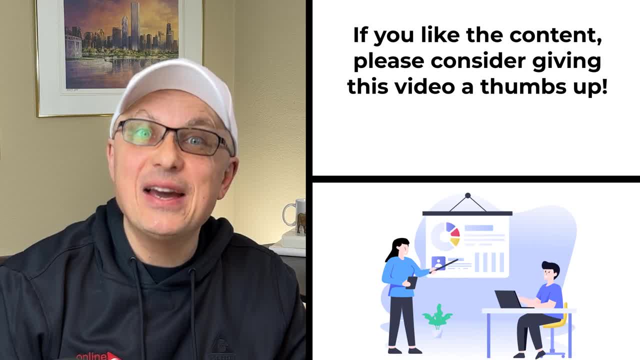 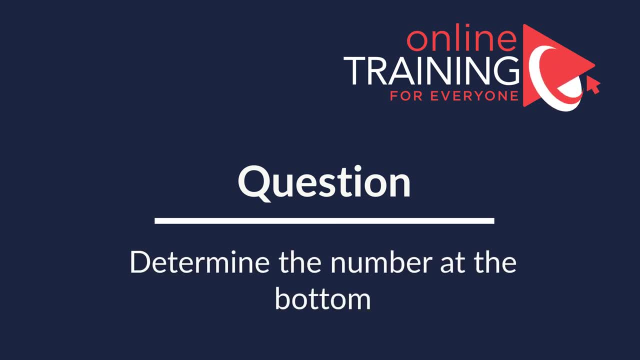 and we will make sure you will get it in the future. And now let's continue and get you ready for the test. Here is an interesting question about how to determine dice's number. at the bottom, Dice was rolled twice and dice's numbers. 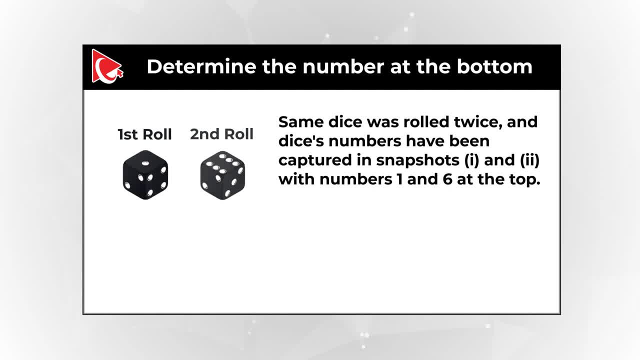 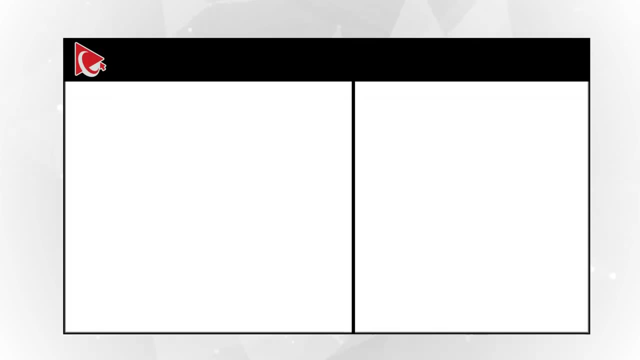 have been captured in snapshots 1 and 2, with numbers 1 and 6 at the top. The dice was rolled again. You need to determine the number at the dice's bottom, if number 5 is currently at the top. You have four different choices. 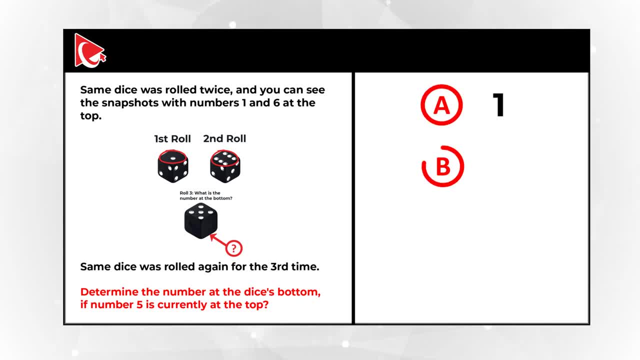 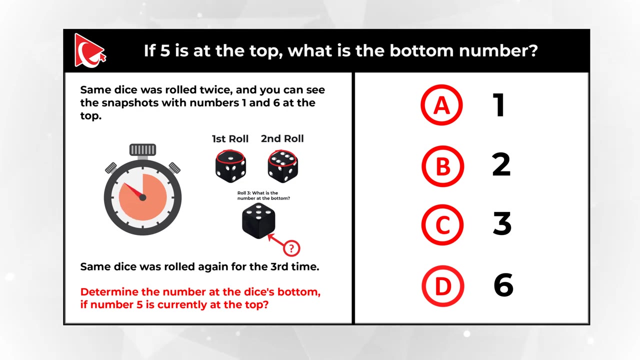 Choice A: 1, 2, 3, 6. Do you see the answer? Please take a close look because the answer may not be obvious. Maybe pause this video to give yourself a little bit of time to find the solution. Are you ready? 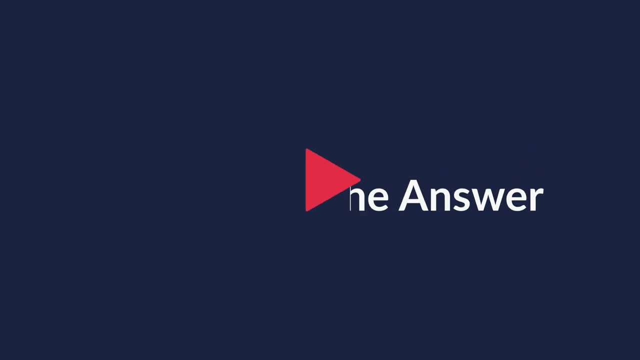 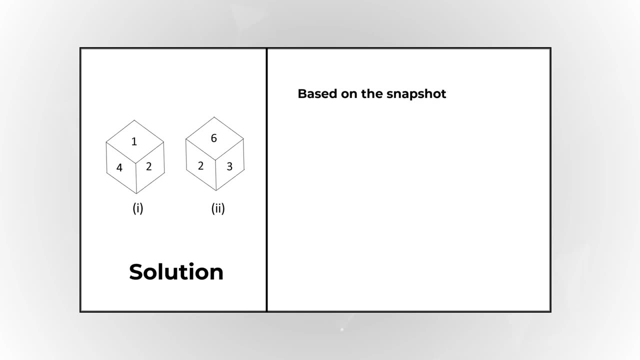 Let's move forward and get to the correct solution together To solve this challenge. let's look at the dice's snapshots. Based on both snapshots, we can learn that numbers 4,, 1,, 3 and 6 are all adjacent to number 2.. 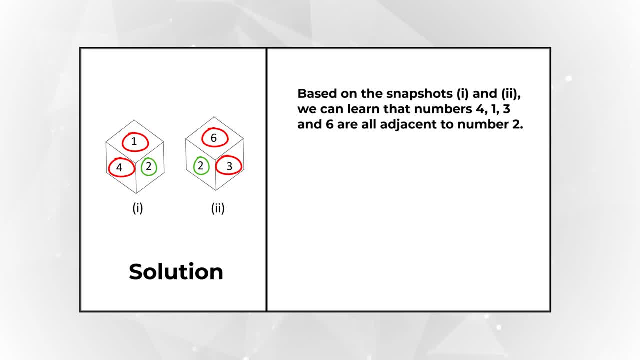 Because dice only has six sides and correspond in six numbers. based on the two snapshots, we can determine that 5 must lie opposite of number 2.. This is why if 5 is at the top, then 2 must be at the top. 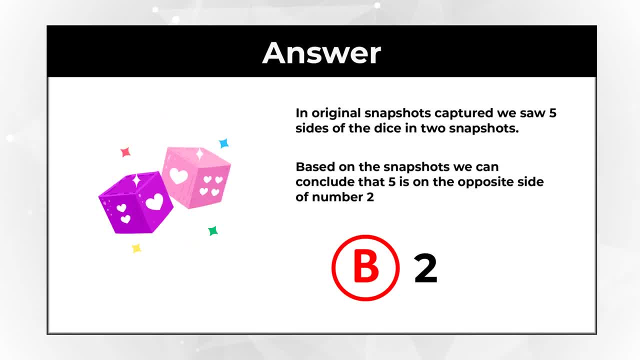 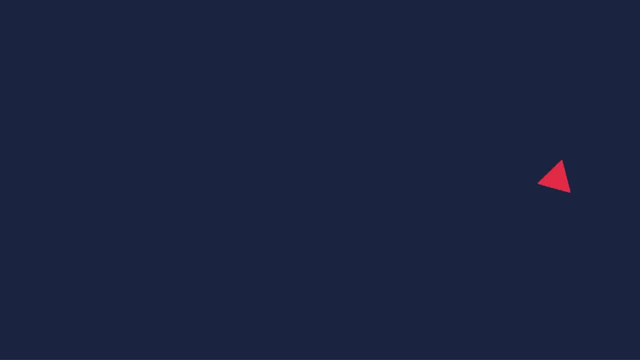 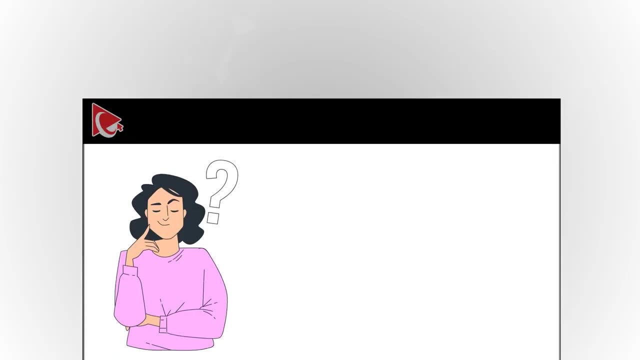 Did you figure it out on your own. Please share your thoughts and the way you solved this challenge in the comment section of this video. Here is a very interesting question, which may not be as simple as it looks. You are presented with the sentence: Scientists consider something. 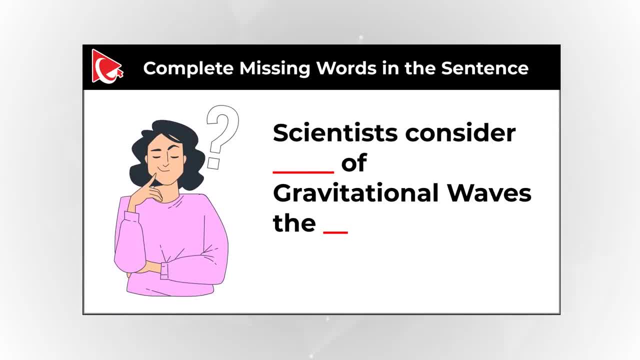 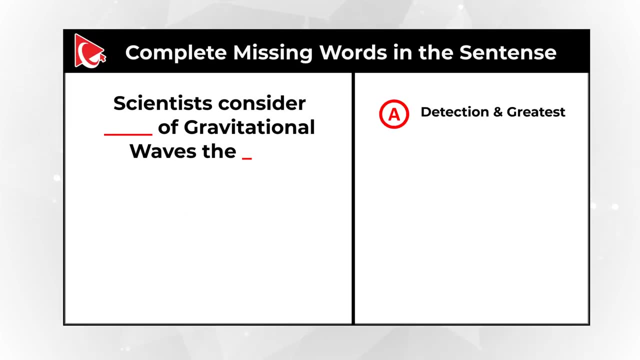 of gravitational waves, the discovery of the 21st century. You need to complete missing words and replace something in the sentence in order to solve it. The answer is one out of four different choices. Choice A- Detection. and greatest Choice B- Energy-caring and amazing. 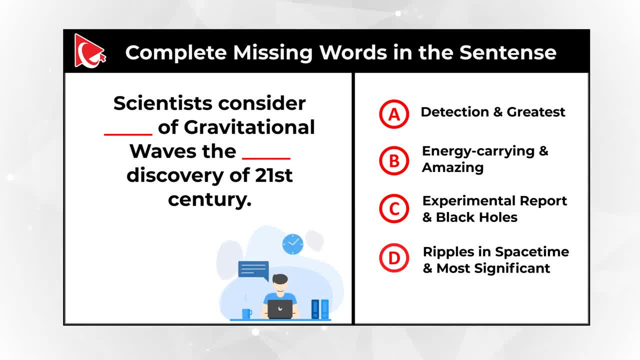 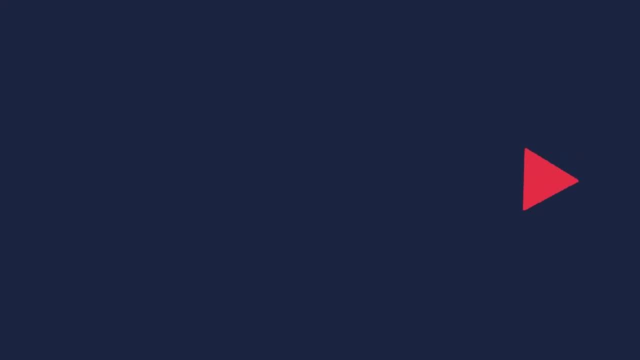 Choice C: Experimental report and black holes. and Choice D: Ripples in space-time and most significant. Give yourself a little bit of time, maybe 10 to 15 seconds. Feel free to pause this video and answer. As you might have figured out, the answer here is choice A. 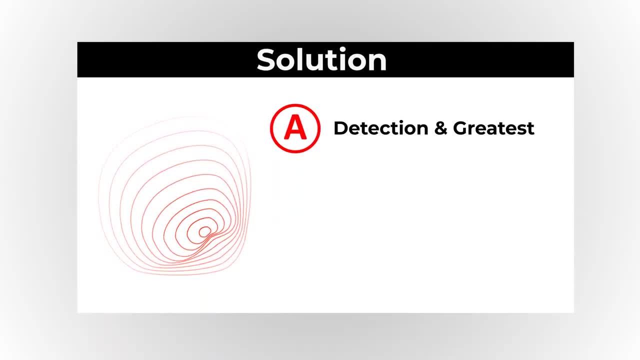 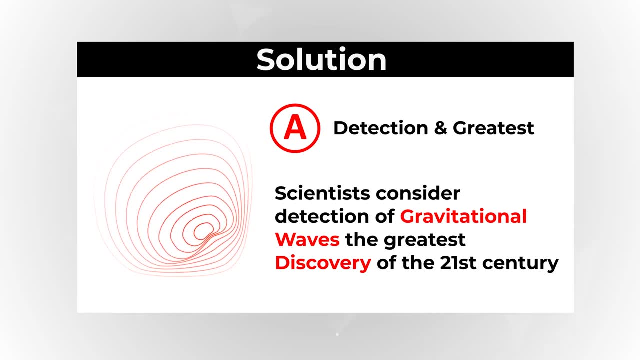 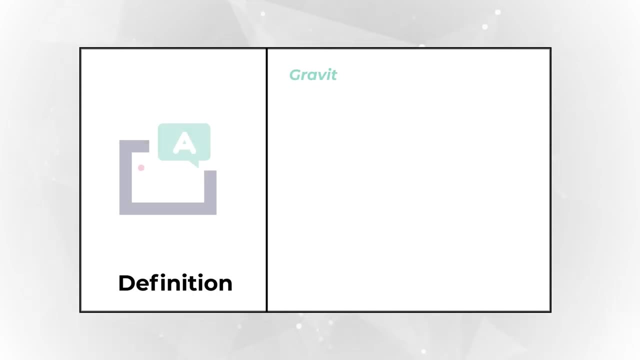 Detection and greatest. Let's look at the full sentence. Scientists consider detection of gravitational waves the greatest discovery of the 21st century. To better understand the magnitude of the discovery, let's look at the definition of gravitational waves. Gravitational wave is an energy-carrying wave. 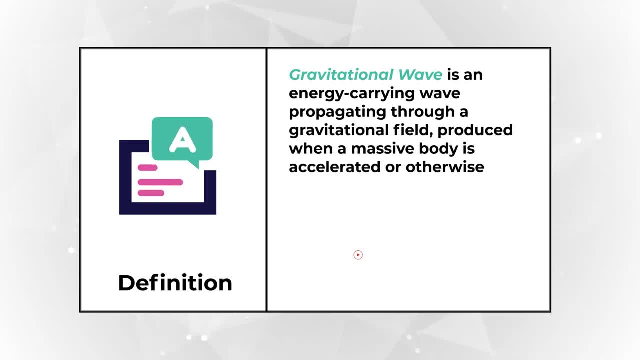 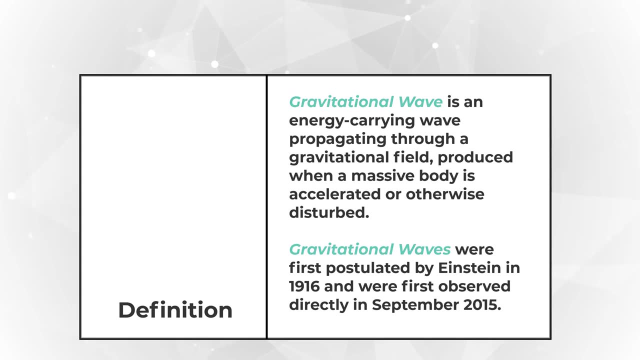 propagating through the gravitational field produced in a massive body of accelerated or otherwise distributed Gravitational waves were first postulated by Einstein in 1916 and were first observed directly in September of 2015.. The cool thing about this particular problem is that to solve it. 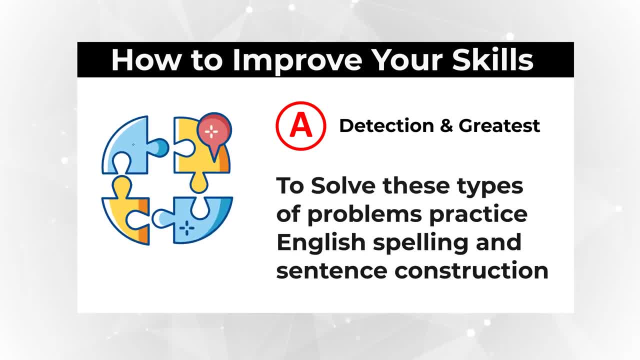 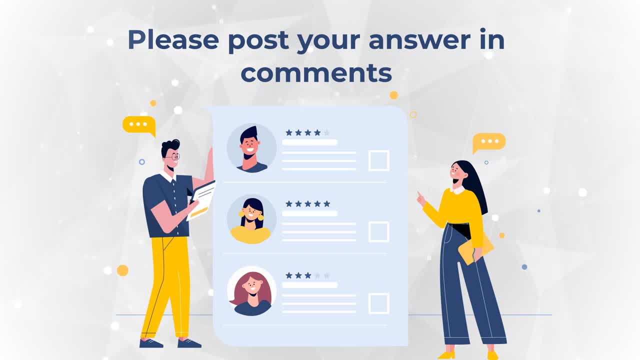 you don't need to know much about gravitational waves, but you need to know how to form English sentences. Hopefully you've nailed this question, reconfirmed your knowledge and now know how to answer similar problems on the test. Here's an interesting question. you might easily get on the test. 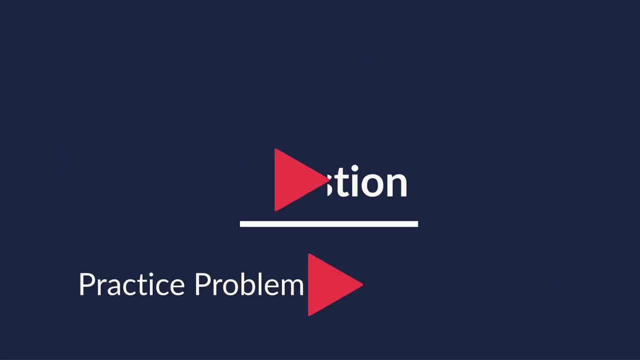 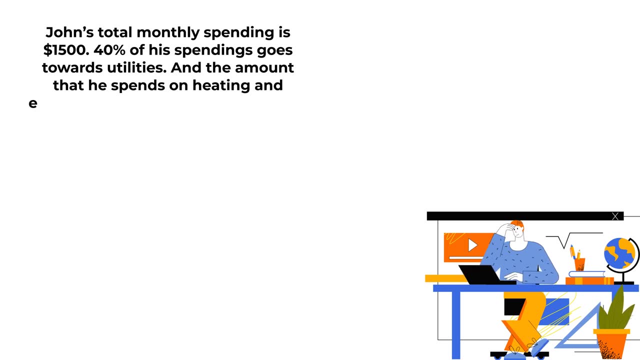 John's monthly spending is $1500.. 40% of his spending goes toward utilities and the amount that he spends on heating and electricity is 15% more than what he spends on utilities. How much does John spend on things besides heating electricity? 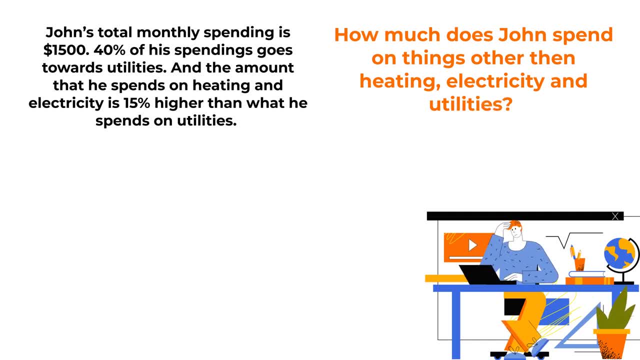 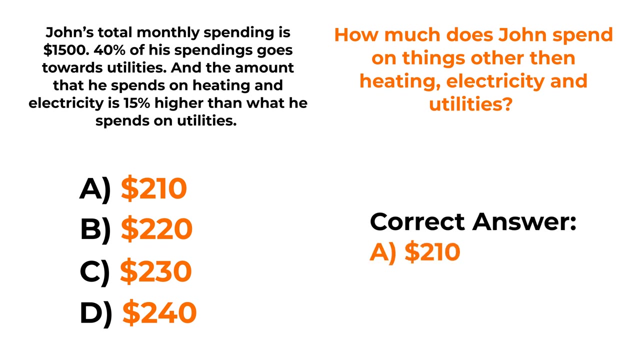 and utilities. You're presented with four different choices: Choice A- $210, Choice B- $220, Choice C- $230 and Choice D- $240. Do you see the answer? Give yourself a little bit of time to see if you can calculate the solution. The correct answer here is: 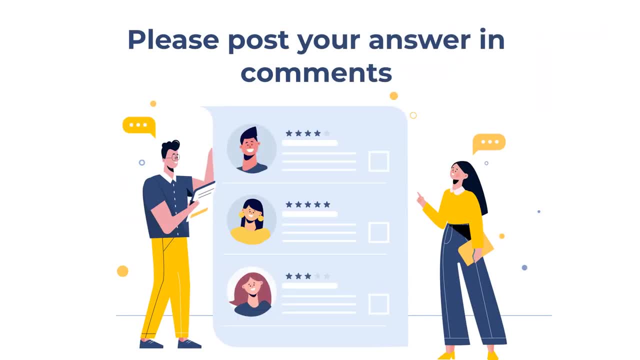 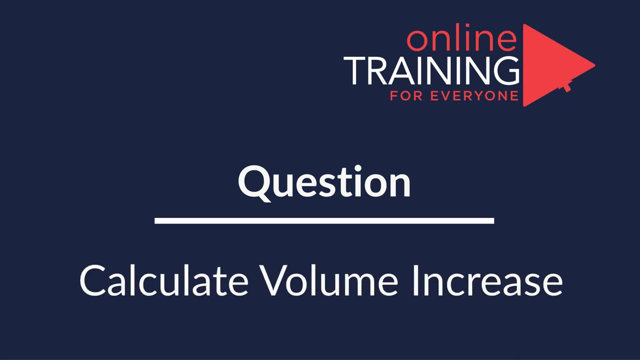 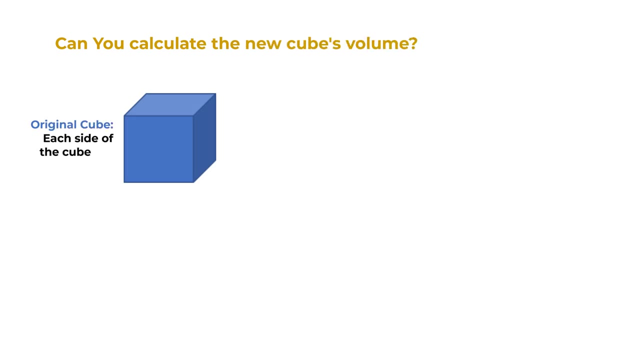 Choice A $210. Do you know how to get to this answer? Good luck, Here's a very interesting question we frequently see on the test. A 5x5x5 cube has its sides length increased by 40% As a result of these changes. 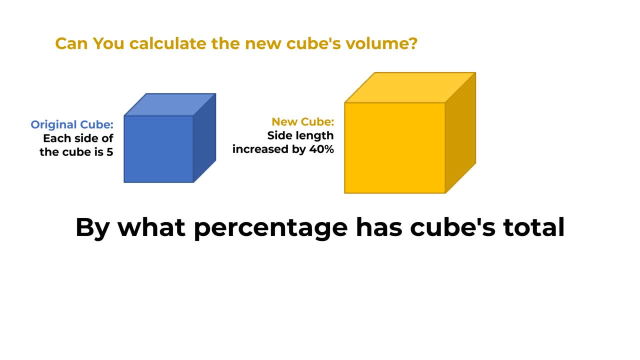 by what percentage has cube's total volume increased? You're presented with four different choices: Choice A- $274, Choice B- $325, Choice C- $379 and Choice D- $379. Do you see the answer? Give yourself a little bit of time, because the answer to this question